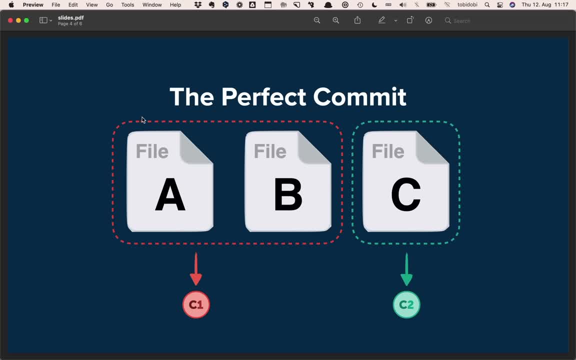 The bigger a commit gets, the more topics that are mixed into the commit, the harder it gets to understand, both for your colleagues and for yourself in the future. So Git's staging area concept is really helpful in this context. It allows you to select specific files or even parts of those files for the next commit. 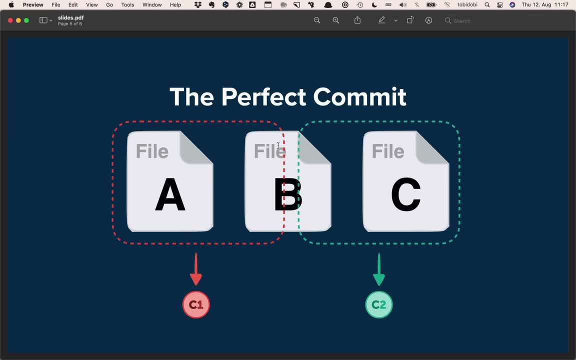 So this is what the staging area can do for you. You can really select individual files for one commit and even parts of files. For example, you can select a single file for one commit and leave others for a future commit. So let's take a look at a practical example. 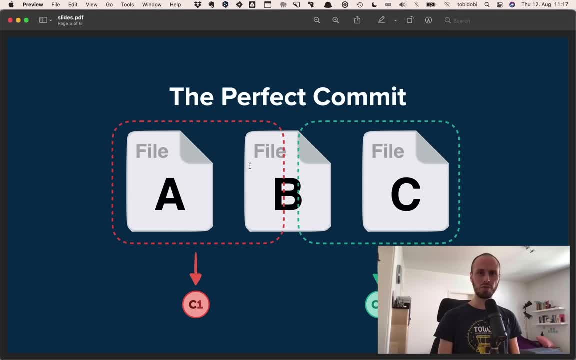 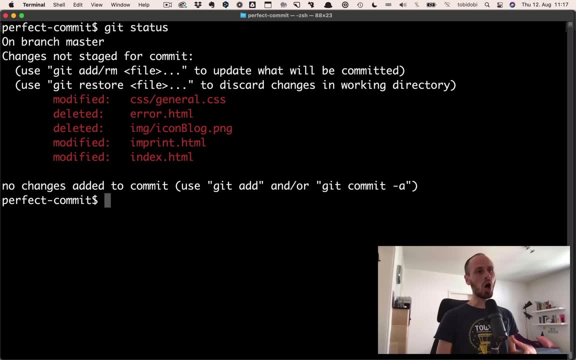 And over the last few hours, or maybe even days, we've created a bunch of changes. Let's say Git status here, But let's say that not all of those are about the same topic. So let's stick to that golden rule of version control to only combine changes from the same. 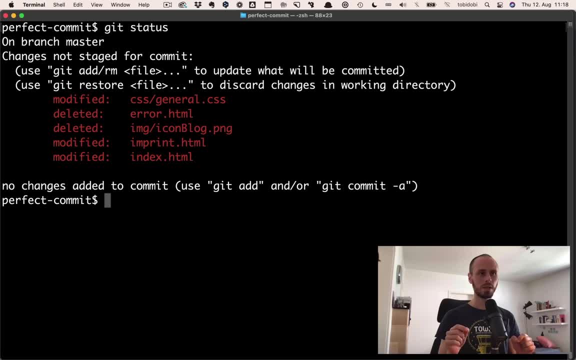 topic in a single commit And you probably already know that to include a specific file we can simply type git add and the name of the file. So let's add that CSS file here And voila. And let's take a closer look at another file- index HTML- and see what changes it currently. 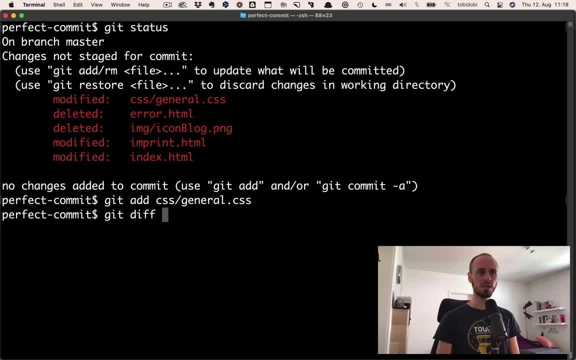 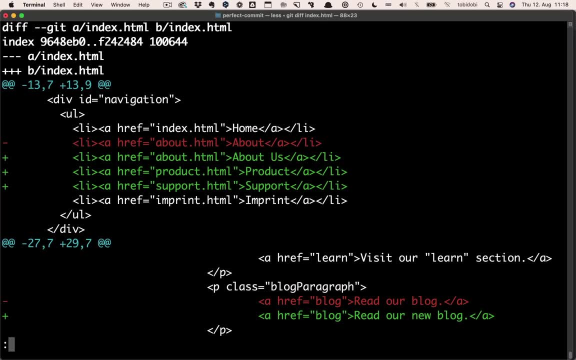 contains. So we can use git diff for that. And we can see that there are two parts Or chunks of changes at the moment, And let's say that the first one belongs to the next commits topic but not the second one. So let's just add the first part to the staging area. 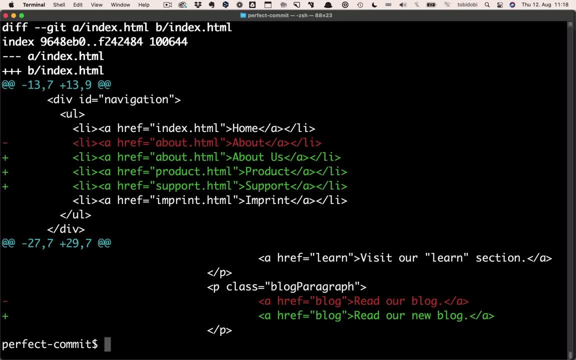 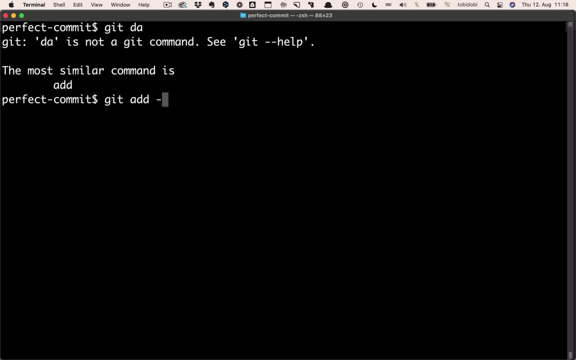 We can do that. I mean just exit the output here. We can do that with the git add. Git add dash P flag P brings us down to the patch level. we want to decide on the patch level, what to include and whatnot. 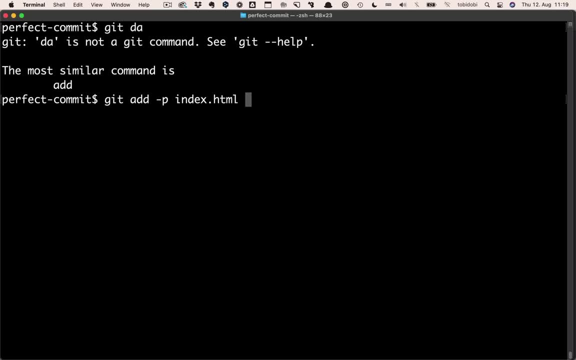 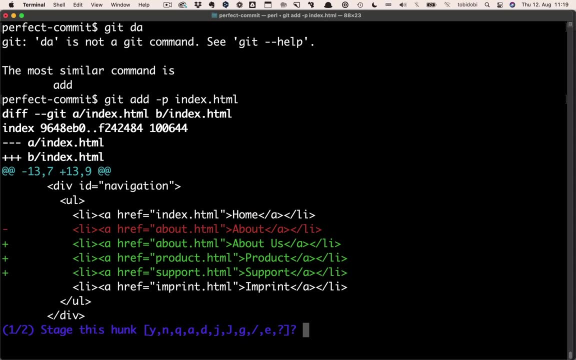 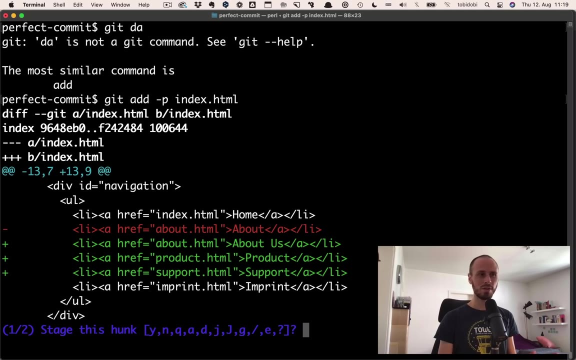 And we want to do that with index HTML. So now git steps through every, every single chunk of changes with us And it asks us a simple question: Do we want to add this chunk or hunk to the staging area or not? Don't worry about all the other possible answers you can give in that situation. 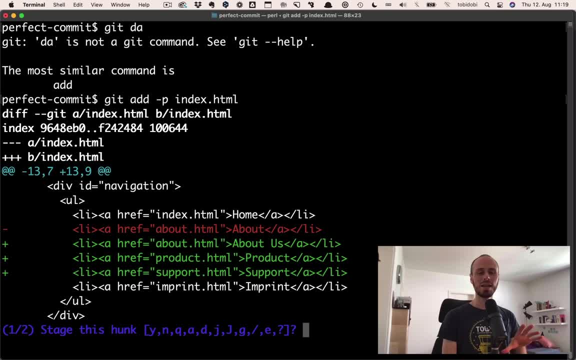 I don't know them. I don't want to sleep at night. For us, a simple Y for yes or N for no is sufficient. So let's say: this one is actually the topic that we want to commit. So let's say yes, we want to include that. 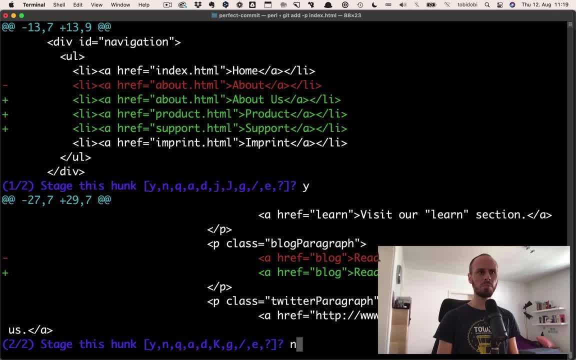 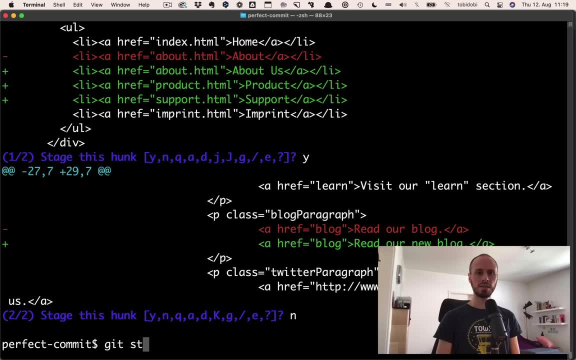 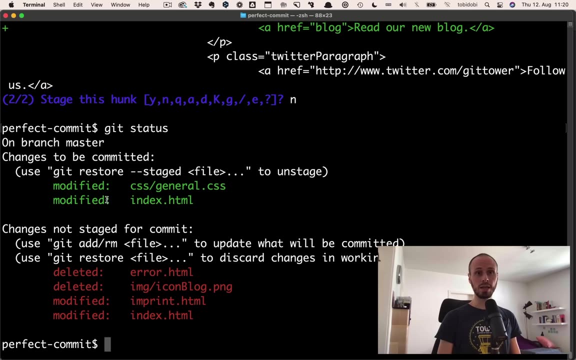 And and. for the second one, this is not the same topic, So let's leave that out of the staging area for the moment. So if we now take another look at git status, we can see that parts of index HTML will be included in the next commit: changes to be committed and other parts. 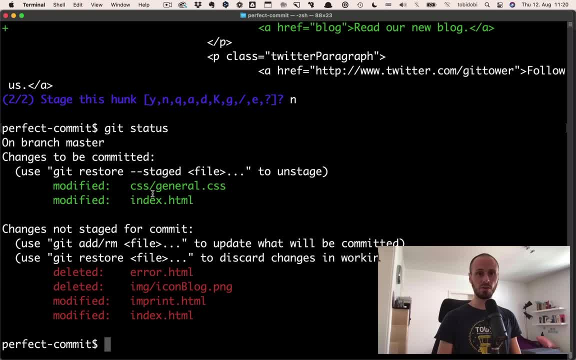 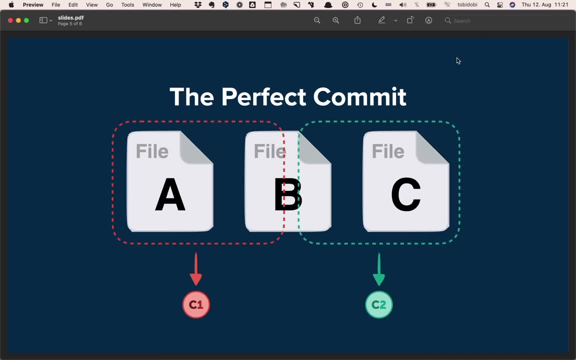 will be left for a future commit Again, so index HTML is listed twice Awesome. Crafting a commit like this in a very granular way will help you create a very valuable commit history, one that is easy to read and to understand, And this is crucial if you want to stay on top of things. 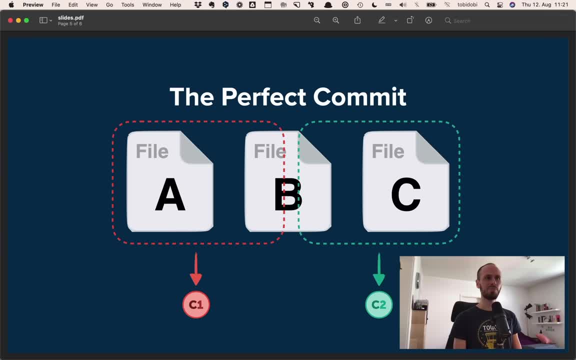 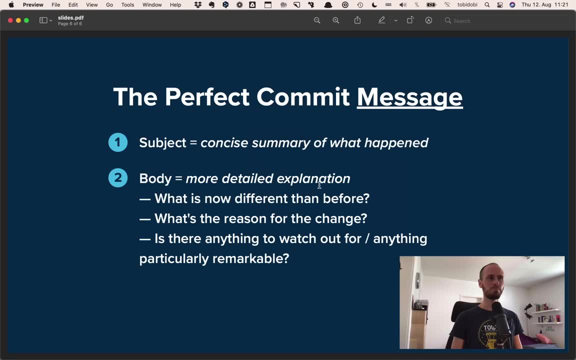 Now let's talk about the second part of creating that perfect commit And that is providing a great commit message. We'll start with the subject line. So of course conventions are different between teams, But generally the advice is to write something very concise. 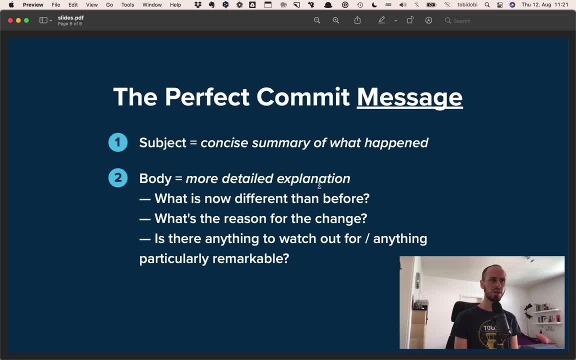 less than 80 characters if possible, And the subject should be a very brief summary of what happened. And here's a little hint: If you have trouble writing something short and concise, then this might be an indication that you've put too many different topics into that commit. 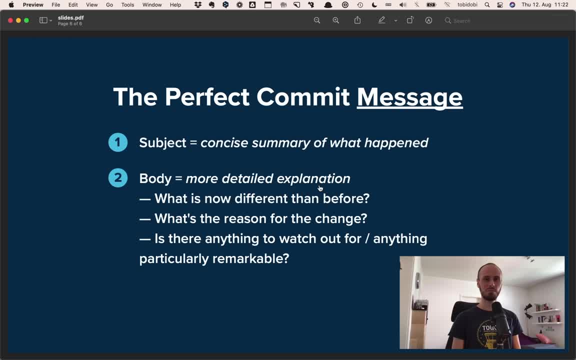 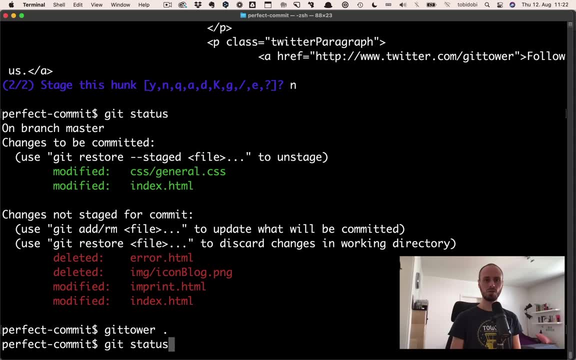 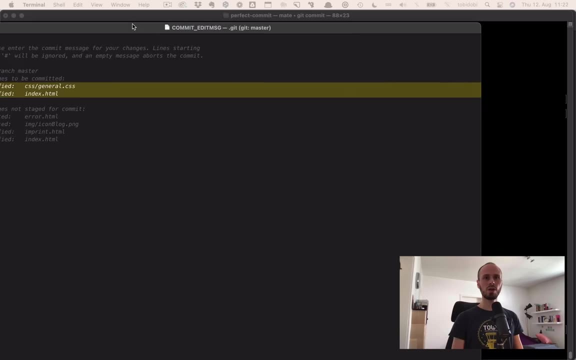 Right, So let's go to the command line And if I now type so, I have a couple of changes again staged for the next commit. If I type git commit, I will get an editor window where I can enter a commit message. 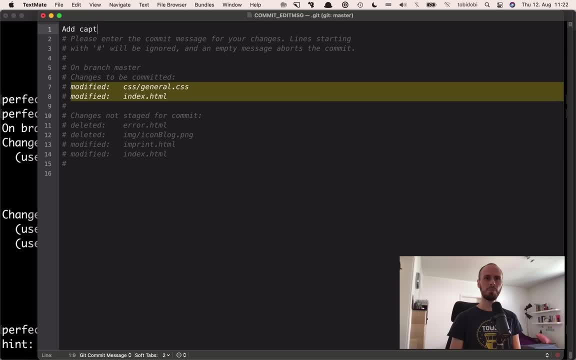 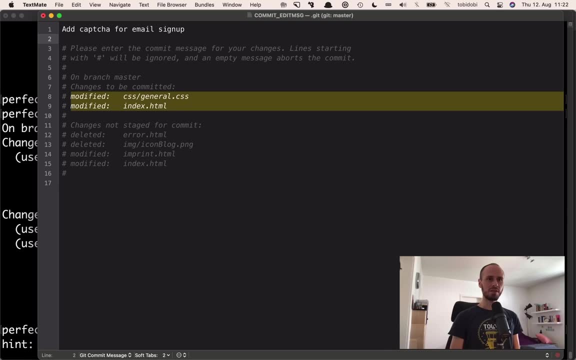 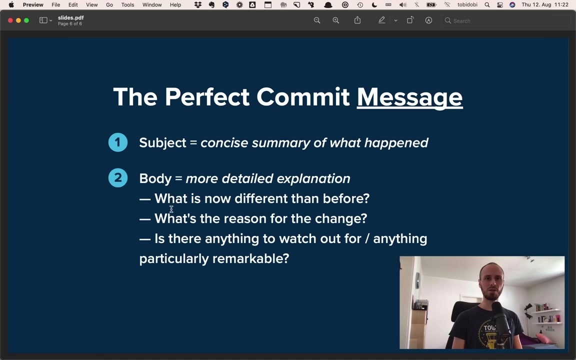 And we'll write something simple: Add captcha for email sign up. If we add an empty line after the subject, git knows we are writing the body of the message And here's room for a much more detailed explanation. So here are a couple of questions you might want to answer with your commit message body this year. 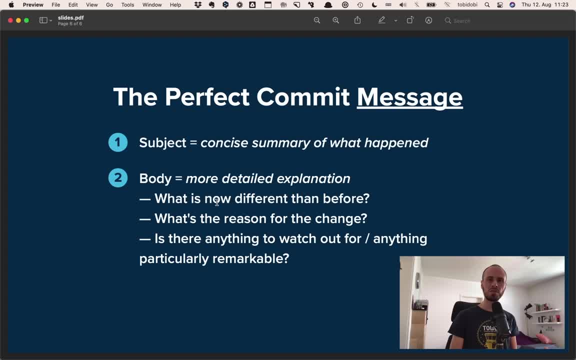 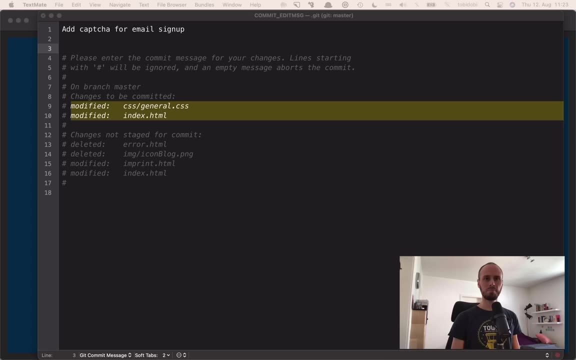 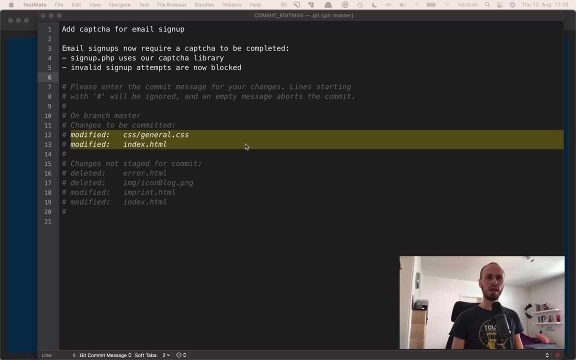 What's now different than before? What's the reason for the change, And is there anything to watch out for Or anything particularly remarkable about that commit? So I'll write my version of that in the text editor here And voila. 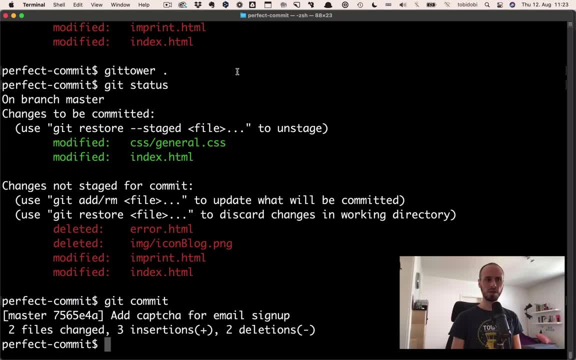 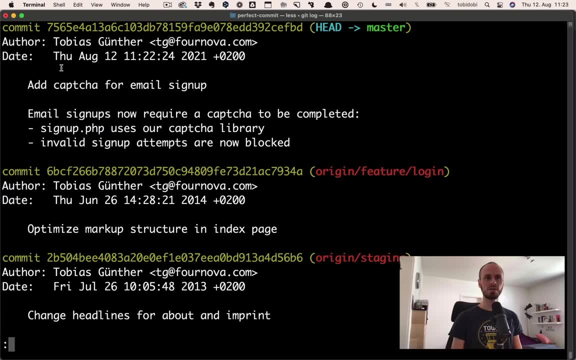 So let's save and close this And the commit is done. Let's take a quick look at git log And we can see: okay, so this is the last commit we just did. This is the subject And this is the body of the message. 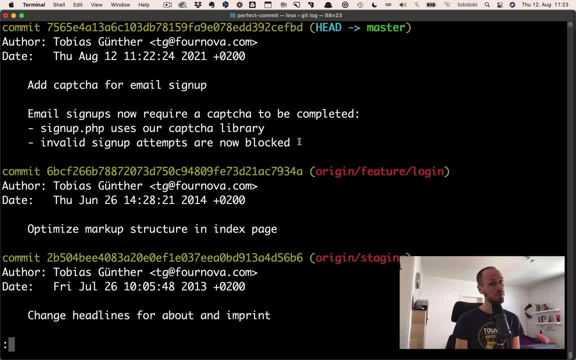 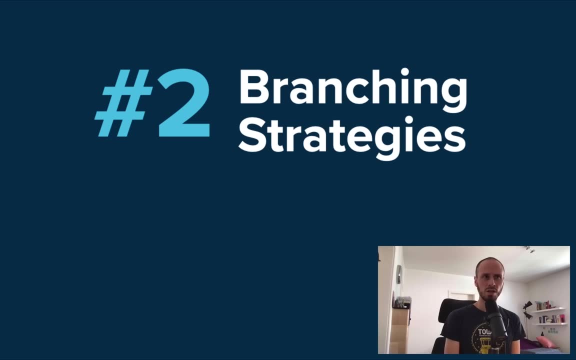 So by answering these questions, you're doing your colleagues and your future self a huge favor, because it helps to understand what exactly happened in this revision and what to watch out for. Let's talk a bit about branching strategies. This is an important topic because git leaves it completely up to you how you want to work. 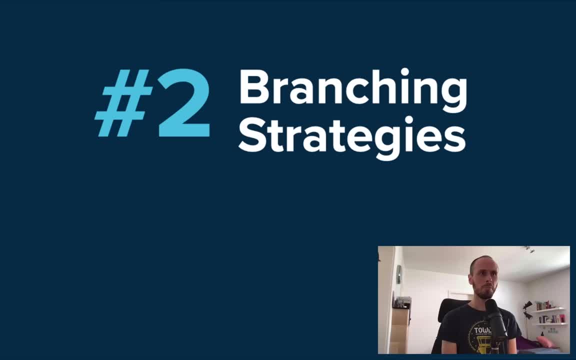 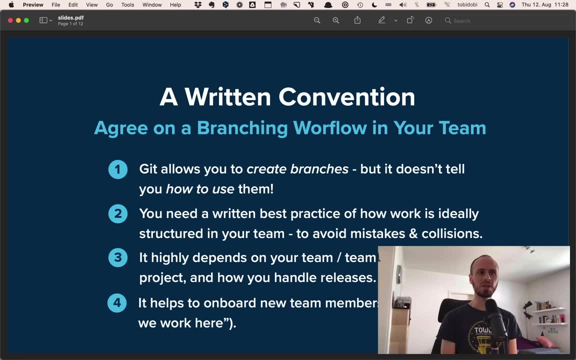 with branches. Git only provides the tool, but you and your team are responsible for using it in the optimal way. And this brings us to our first topic: conventions. If you work in a team, you need to come up with a clear convention on how you want to work with branches. 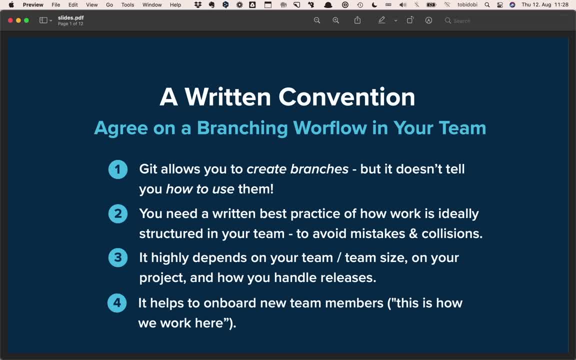 And you need to write this down somewhere where it's accessible to everyone. Why your team needs a written convention, you ask Because git allows you to create branches, but it doesn't tell you how to use them. You need a written best practice of how to work, or how work is ideally structured in your team, to avoid mistakes. 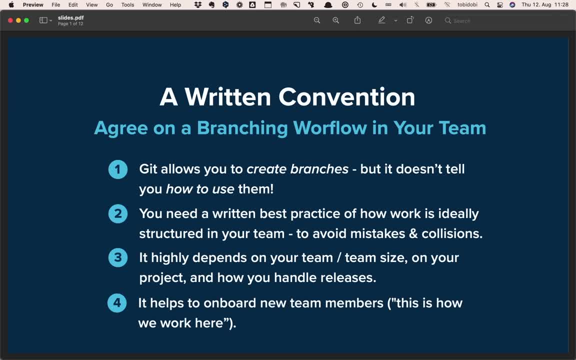 If you want to work with branches, you need to know how to work with branches. and you need to know how to work with branches And this depends on your team and team size, on your project and how you handle releases of your software. 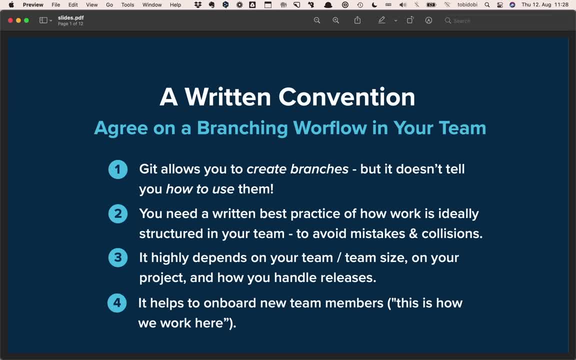 Last but not least, it helps to onboard new team members. When new people join your team, you can point them to your documented convention and they'll quickly understand how branches are handled in your team. When you think about how you want to work with branches, you automatically think about 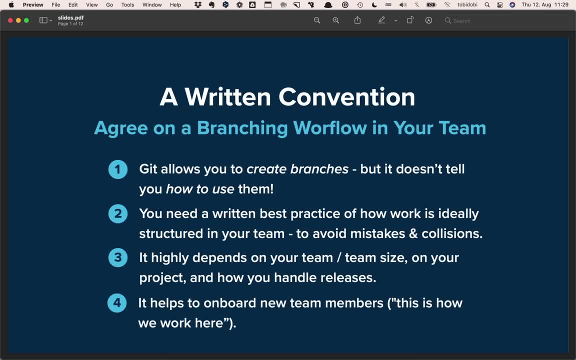 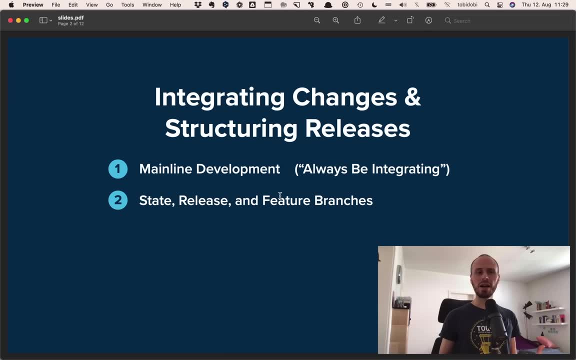 how you integrate changes and structure releases. these topics are tightly connected. To help you better understand your options, let's simplify a little bit. I'll show you how- two extreme versions of how you could design your branching workflows, And the motto of the first one is always be integrating the mainline development. 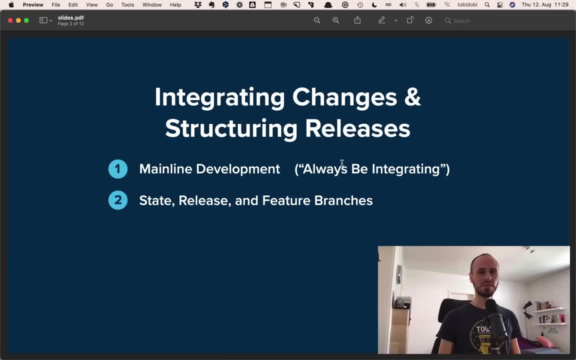 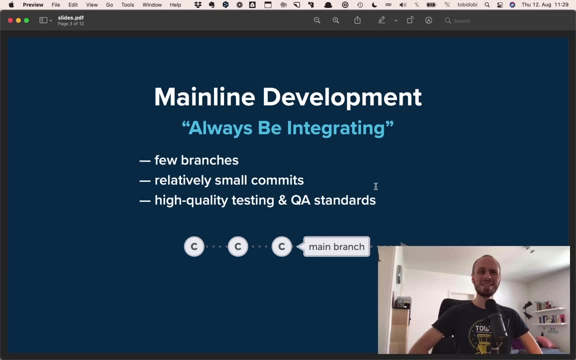 Always integrate your own work with the work of the team. That's the motto here, And so this is how it could look. In this example, we only have a single branch where everyone contributes their commits, So this is a really simplified example. I doubt that any team in the 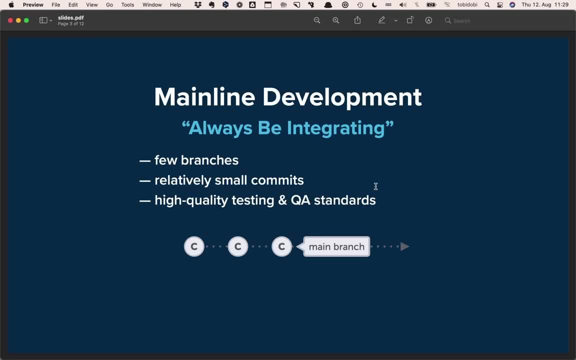 real world would have such simple branching structure. But for illustration, this extreme simplified example helps us understand the advantages and disadvantages of this model. So in an always be integrating model you have very few branches And this makes it easier to keep track of things in your team. 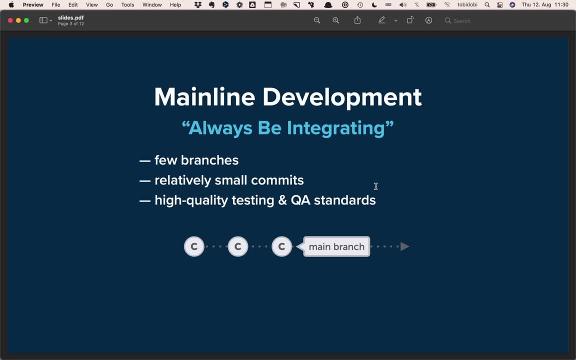 Your project, of course also commits in this model must be relatively small. This is a natural requirement because you cannot risk big, bloated commits in such an environment where things are constantly integrated into production code, And this also means that you must have a 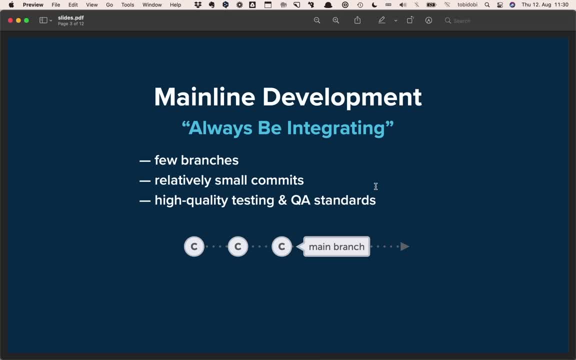 high quality testing environment set up. Again. the premise in this model is that code is integrated very quickly into your mainline, your production code, And this means that testing and QA standard in your team must be top notch. If you don't have this, this model will not work for you. 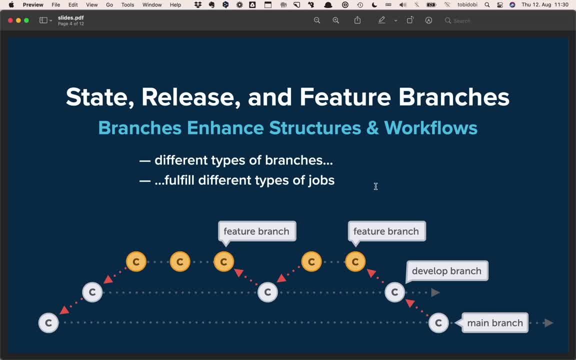 The other end of the spectrum is when multiple different types of branches enter the stage. So here branches are used to fill, to fulfill different jobs, new features and experiments are kept in their own branches. releases can be planned and managed, managed in their own branches and even different states in your development flow, like production. 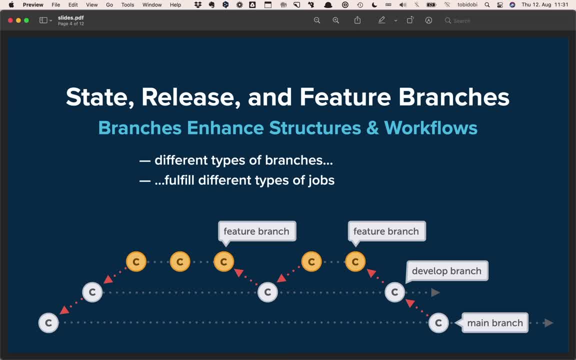 can be represented by branches. Remember that this all depends on the needs and requirements of your team and project. It's hard to say that one approach is better than the other, And although a model like this one seems complicated, it's mostly a matter of practice. 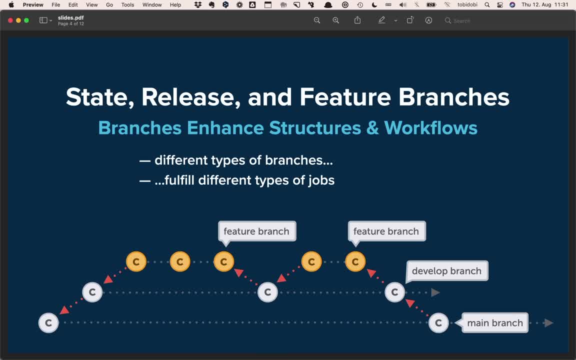 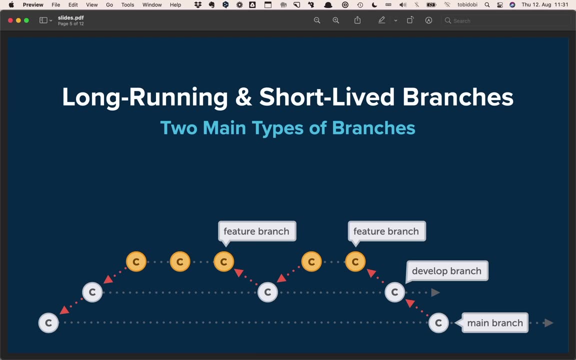 and getting used to it And, as I already said, in reality most teams are working somewhere in between these extremes. Now let's look closer at two main types of branches and how they are used. These two types of branches are long running and short lived branches. So the distinction 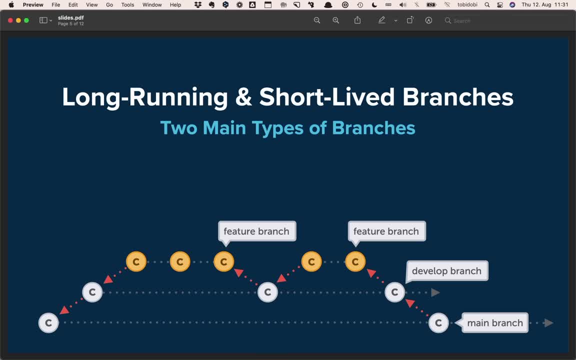 between a long running and a short lived branch is one of the broadest you can make, and a very helpful one. So let's start about talking about the long running branches first. Every Git repository contains at least one long running branch, typically something called main or master. But 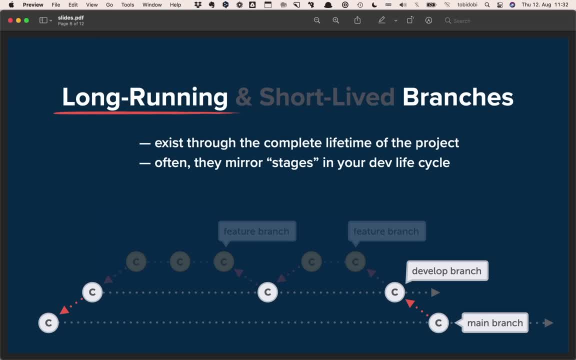 there might be also other long running branches. For example, if you have a long running branch, you might have long running branches in your project, something like develop or production or staging, For example. these branches all have something in common: they exist. 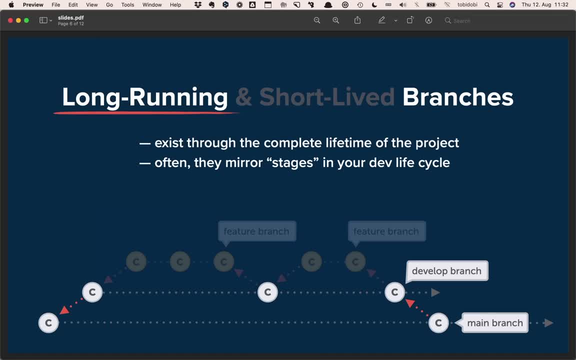 throughout the complete lifecycle of the project. I've already mentioned one typical example of such a long running branch. Every project has a mainline branch, like master or main, And another type of long running branches are so called integration branches, often named develop or 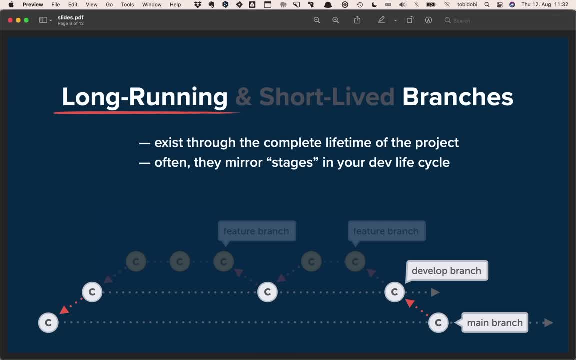 staging. Typically these branches are long running branches, but they're not long running. The long running branches represent states in a project's release or deployment process, If your code moves through different states, for example, from development to staging to production. 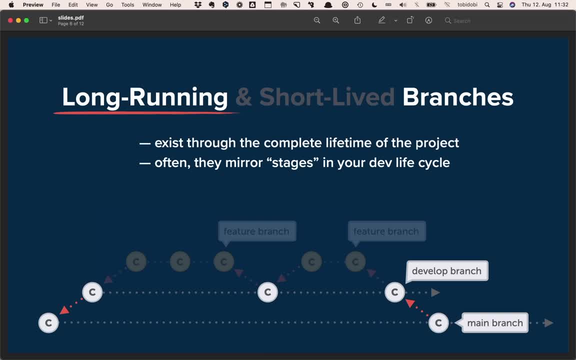 it makes a lot of sense to mirror this structure in your branches too. And finally, many teams have a convention connected to long running branches. Typically, commits are never directly added to these branches. commits should only make it to the long running branch Through integration. So in this example we have the long running branch for the. 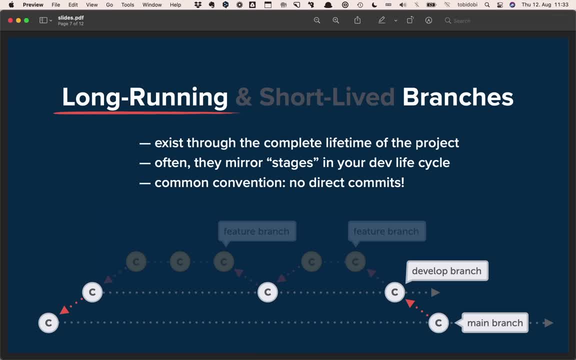 long running branch. In this example, we have the long running branch for the long running branch As we go, the long running branch for the long running branchcomponents, or the long running branch for integration, in other words, through a merge or a rebase. There are a couple of reasons for such. 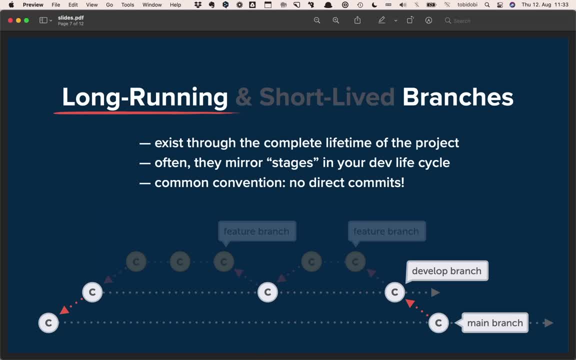 a rule. One has to do with quality. You don't want to add untested, unreviewed code to your production environment as an example, And that's why code should go through different states, tests and reviews before it finally arrives on production. Another reason might be release. 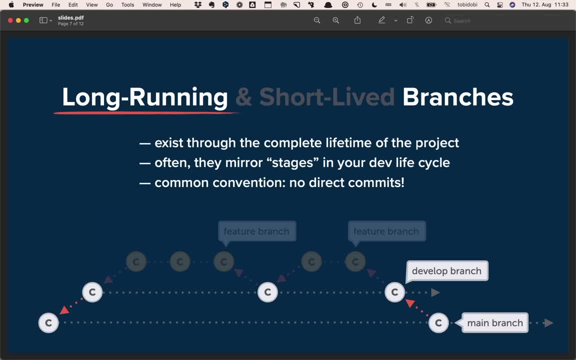 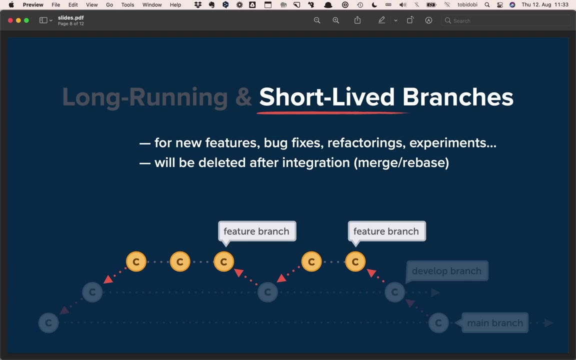 bundling and scheduling, you might want to release new code in batches, maybe even thoroughly scheduled, And without such a rule, when code is directly committed to long running branches like main, keeping an eye on what's released becomes pretty difficult. Now the other type of branches are short lived branches And, in contrast to long running branches, 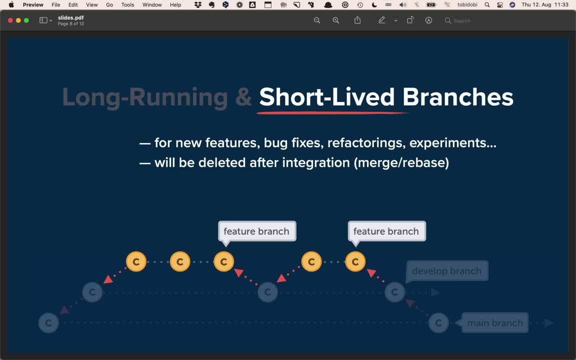 they are created for certain purposes and then deleted after They have been integrated. There are many different reasons to create short lived branches, For example, when you start working on a new feature, a bug fix or refactoring or an experiment, And 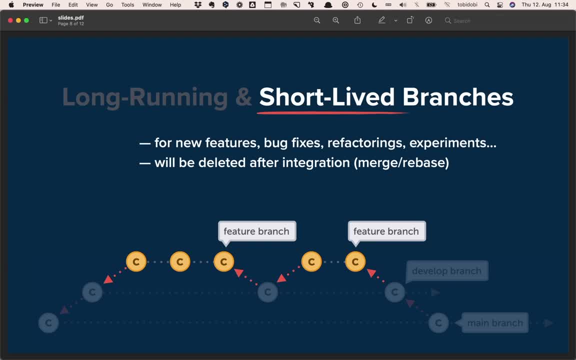 typically a short lived branch will be based on a long running branch. For example, when you start a new feature, you might base that new feature on your long running main branch, for example, And after making some commits and finishing your work, you probably want to reintegrate it back into main. 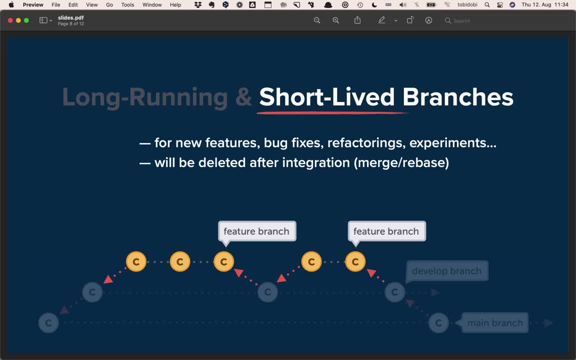 And after you've done that you might want to reintegrate it back into main, And after you've safely merged or rebased it, your feature branch can be deleted, And I've already said that branching strategies will be different for each team and project. It. 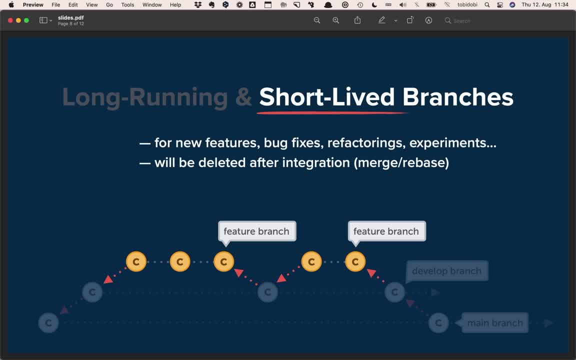 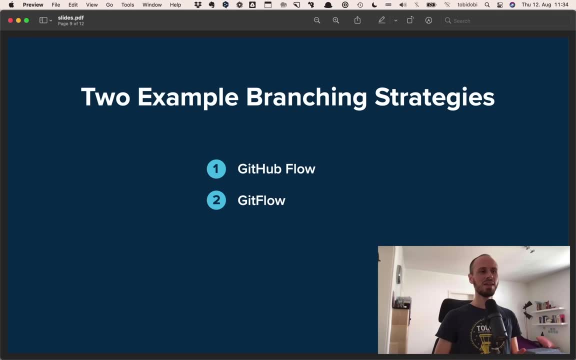 highly depends on your preferences or team size or type of project, But I'd like to give you a glimpse into two pretty popular branching strategies and take both of them as inspiration for your own individual branching strategy. Let's start with GitHub flow. GitHub advocates a workflow that's extremely lean and simple. It only has a single long running. 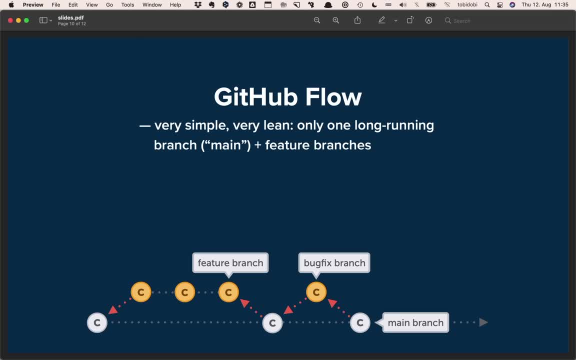 branch, the default main branch, and anything you're actively working on is done in a separate branch- a short lived branch, no matter if that's a feature, a bug fix or a factoring. So this is a very simple, very lean setup. Another very popular model is called Get Flow, And this offers a bit more. 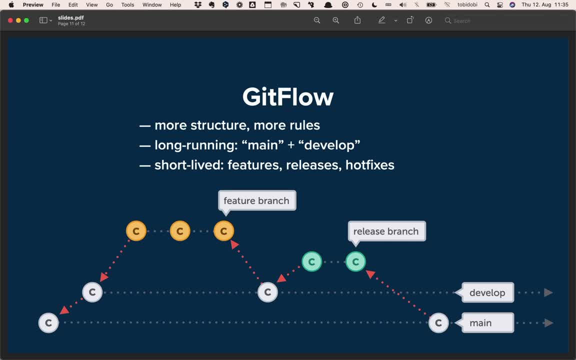 structure but also a little bit more flexibility. This is where a bunch of these features get introduced: structure, but also more rules to follow. So the main branch is a reflection of the current production state. The other long running branch is typically called develop And any feature 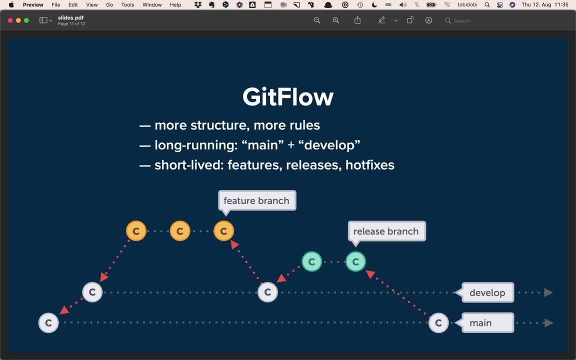 branches start from this one and will be merged back into it. Develop is also the starting point for any new releases. you would open a new release branch, do your testing, commit any bug fixes to that release branch And once you're confident that it's ready for production. 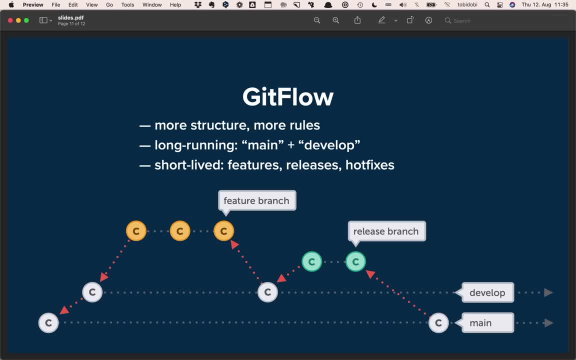 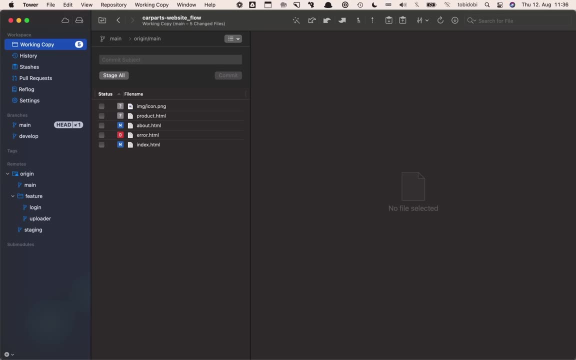 you merge it back into main. you would then add a tag for that release commit on main and close the release branch. As you can see, good flow defines quite a couple of tasks and steps in the process In tower the good desktop GUI that we make. we support users by offering. 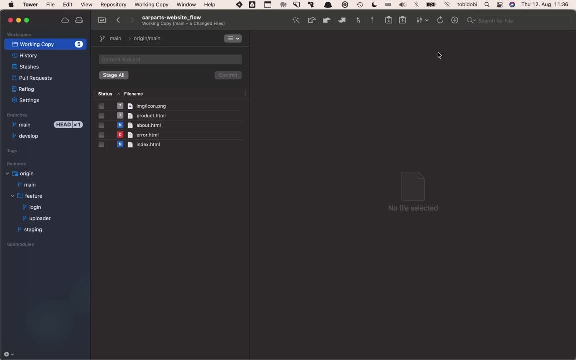 these tasks as shortcuts in the app And that way I can show you here So you have all of the most important actions that get flow brings to you, So you don't have to remember all of the bits and pieces and what you have to do. 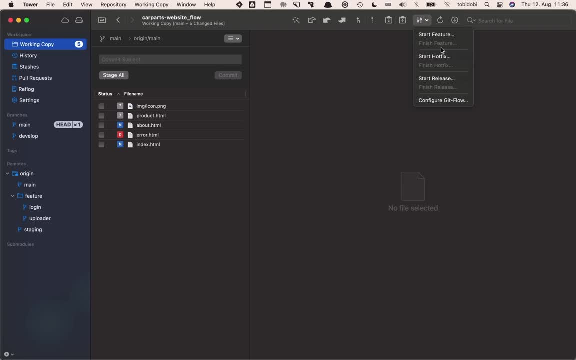 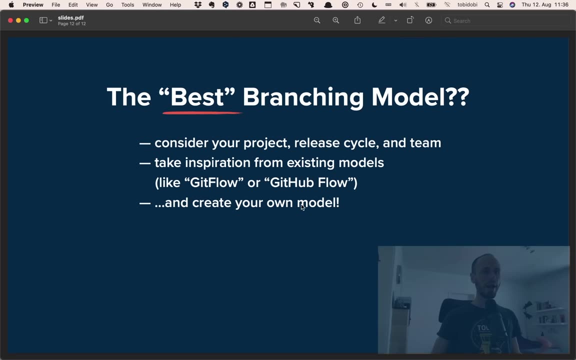 and what comes next that make up these different steps. So if you ask different teams how they are using branches, you will get many different answers. There is no perfect branching model that everyone should adopt. It's more about understanding your project or release workflow and your team and then modeling a branching workflow. 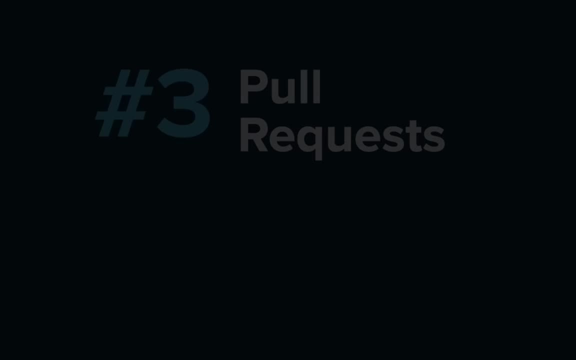 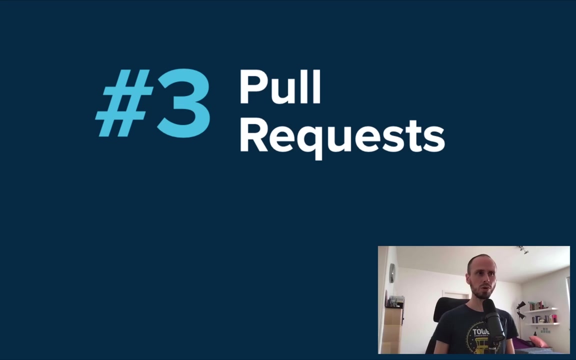 It supports you in the best way possible. Let's talk about pull requests. First of all, you need to understand that pull requests are not a core Git feature. They are provided by your Git hosting platform, which means they work and look a little. 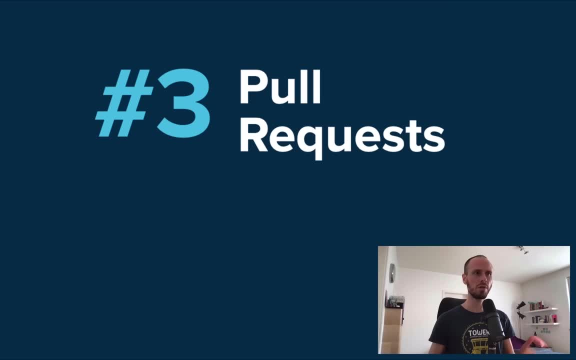 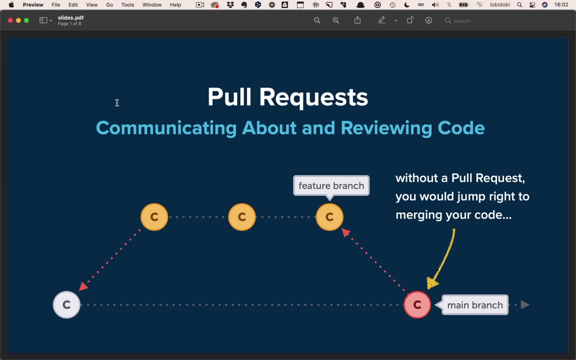 bit differently on GitHub, GitLab, Bitbucket, Azure, DevOps or whatever you're using, But the basic principles and ideas are always the same. It's no longer about why you would want to use pull requests at all. In essence, they are a way to communicate. 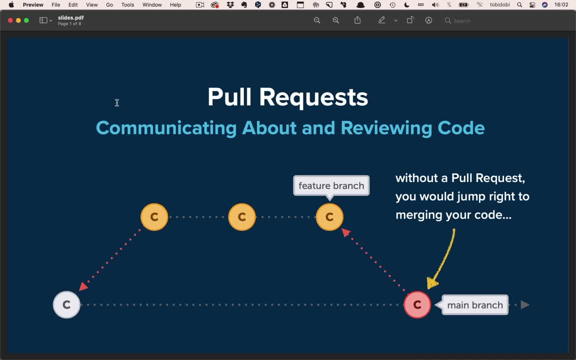 about code and review it. The perfect example is when you've finished working on a feature Without a pull request. you'd simply merge your code into main master or some other branch, And in some cases this might be totally fine. 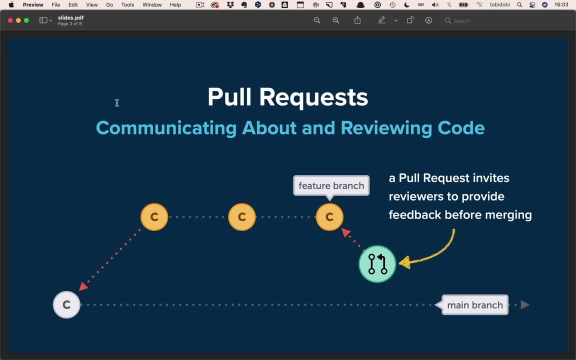 But especially when your changes are a bit more complex or a bit more important, you might want to look in a different direction, And even if you're the one who does that, it's still a problem. So I'm going to hold this up for the next 1 minute before I start your dialogue. 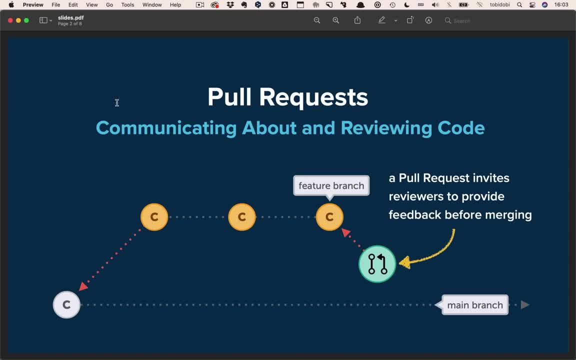 you might want to have a second pair of eyes look over your code, And this is exactly what pull requests were made for. With pull requests, you can invite other people to review your work and give you feedback And, after some conversation about the code, your reviewer might approve the. 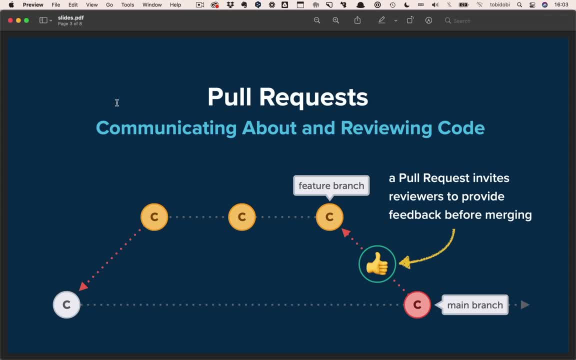 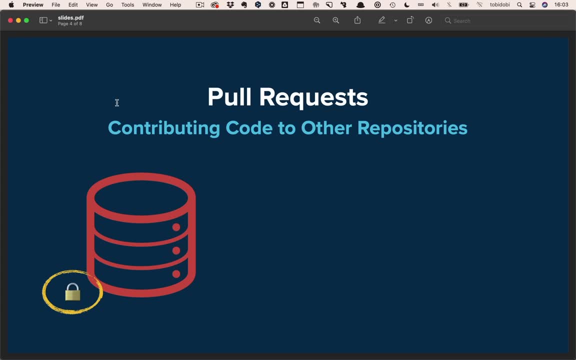 pull request and merge it into another branch. Apart from this, there's another important use case for pull requests. It's a way to contribute to code to repositories which you don't have right access to. Think of a popular open source repository. you might have an idea for improving. 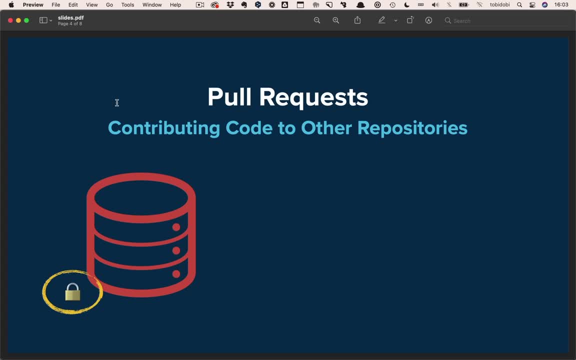 something, but you're not one of the main contributors and you're not allowed to push commits to their repository. This is another use case for pull requests And we also have to talk about forks in this connection. A fork is your personal connection And it's a way to contribute to code to repositories which you don't have right access. 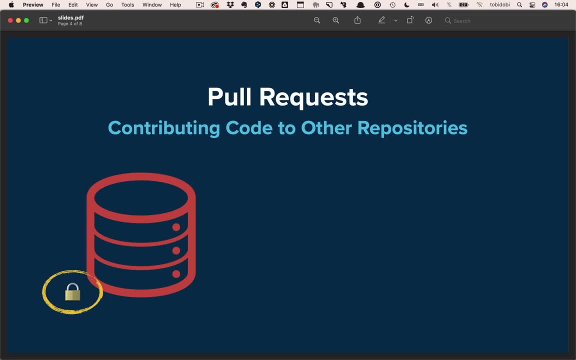 copy of a git repository. And going back to our open source example, you can fork the original repository, make changes in your forked version and open a pull request to include those changes into the original repository, And one of the main contributors can then review your changes and 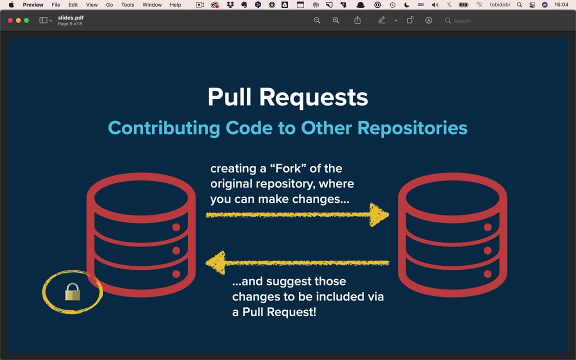 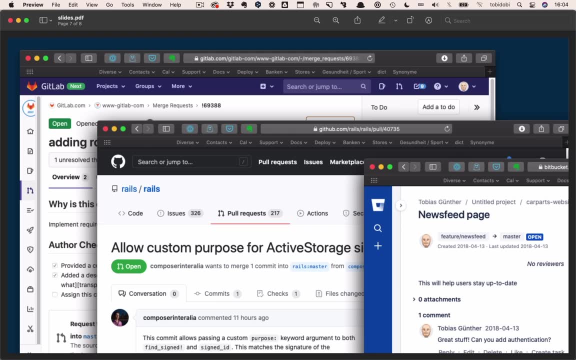 decide to include them or not. I already mentioned it: every git platform has its own design and understanding of how pull requests should work, And they look a little bit different on GitHub, GitLab, Bitbucket or Azure DevOps or whatever you're using. So here as an example, we'll use the GitHub interface. 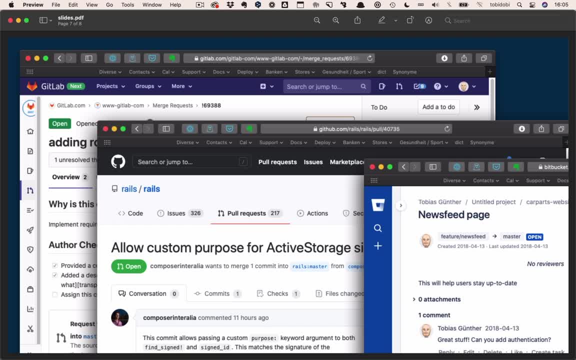 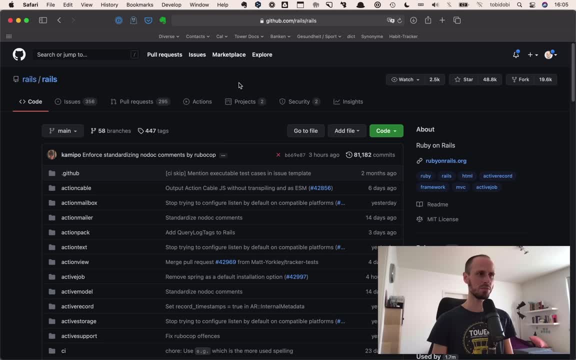 And for this test case, let's use the Ruby on Rails open source repository And let's see All right. so here we're on GitHub on the Ruby on Rails main repository, And in the top right icon you can see that I can fork this repository So I can create my own personal version of the. 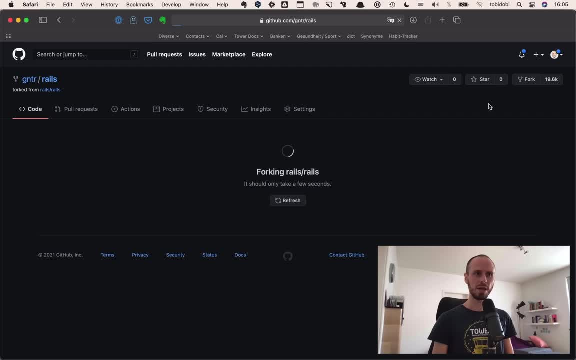 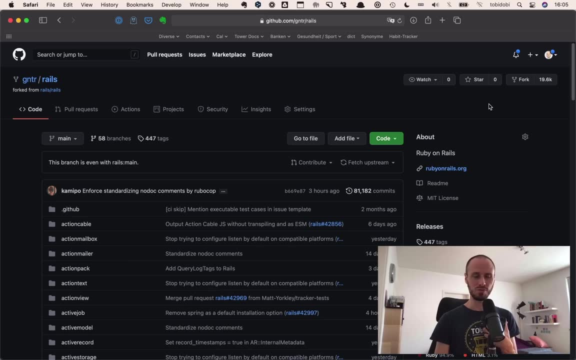 repository And its code base. And again a reminder about why we're doing this: I don't have access to push code into Ruby on Rails, into the Ruby on Rails repository, And for good reasons, of course, because I'm not a Ruby on Rails pro. 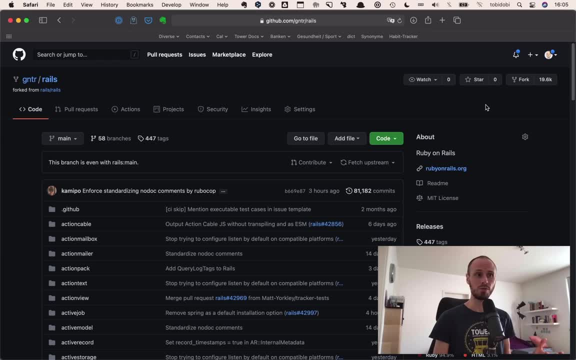 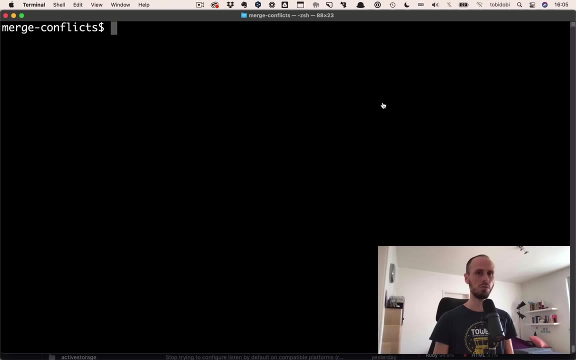 But in my own forked repository changes I can make whatever changes I want. So I just did that. I forked the repository And I can now simply clone that. I'll get the clone URL And then on the command line get clone and remote URL. 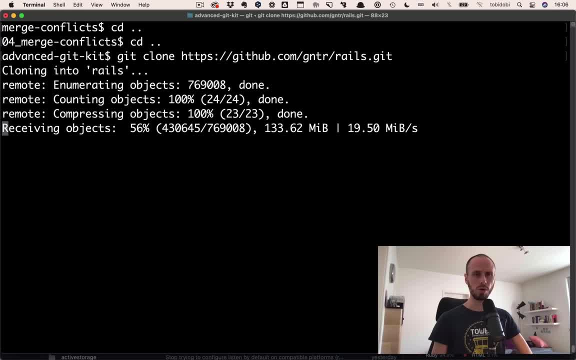 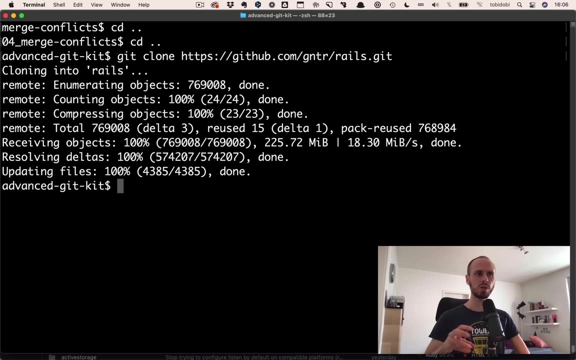 And we will. in a second, when this has finished cloning, we will create a branch and make some changes, So this is also important to understand. pull requests are always based on branches, not on individual commits. So we're creating a new branch which we later request to be included, And let's open. 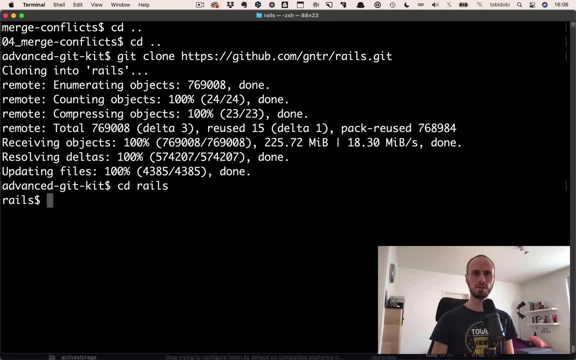 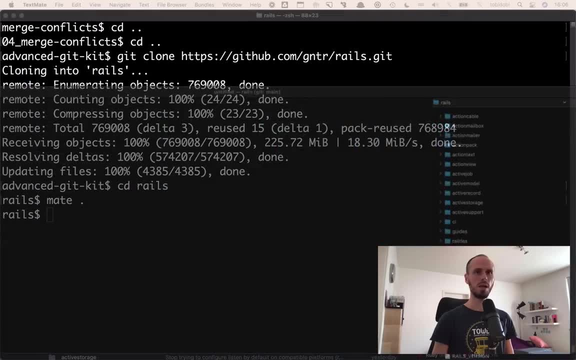 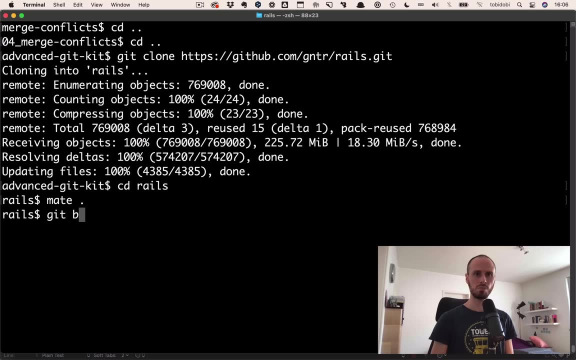 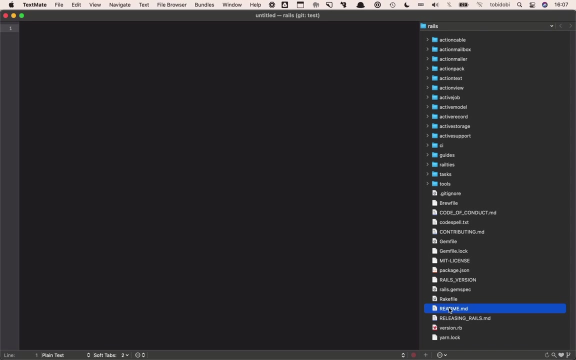 Let's go into rails And open this in my editor And I'll just create a brief branch. get branch test And get checkout test. All right, so I now am on a new branch and can make a silly little change. Let's change something in the readme file. 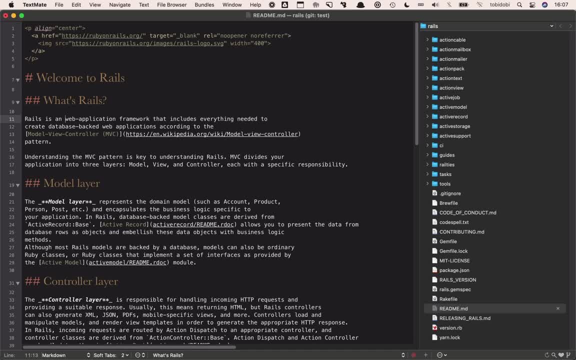 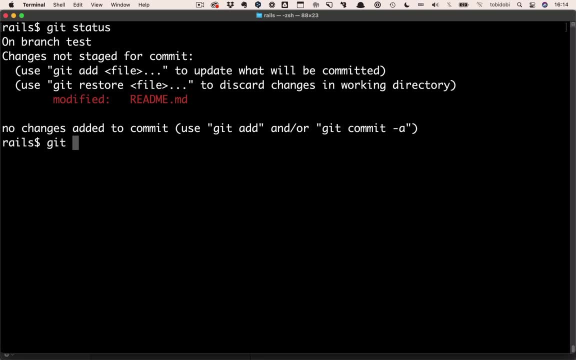 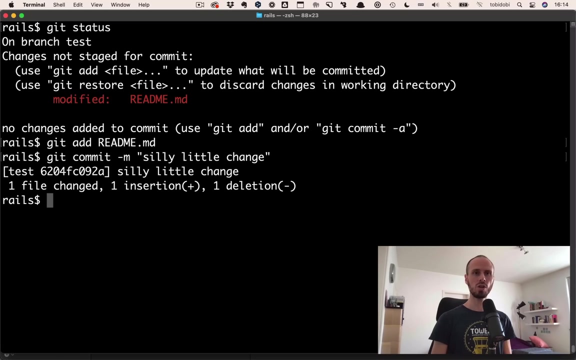 This is a an awesome web application framework. close this. All right, let's take a look at our changes: Get add readme and get commit. dash m silly little change. So we now have made some small changes on a separate branch and we can push that branch to our own remote repository, our fork. So get push. 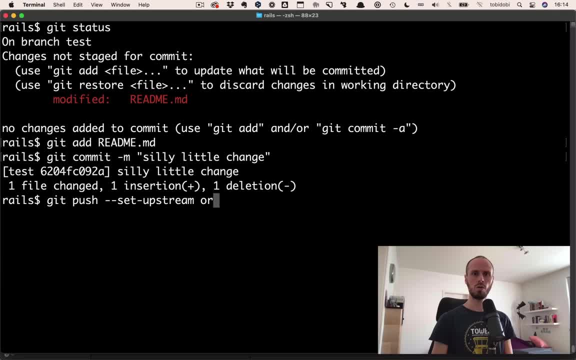 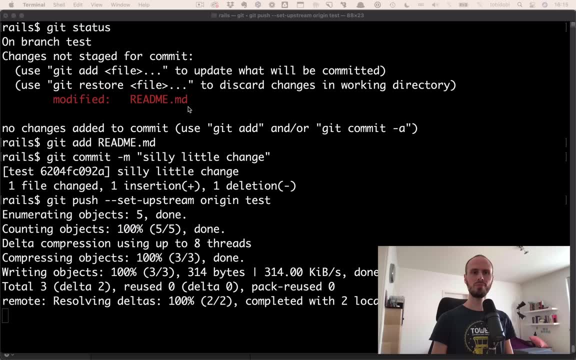 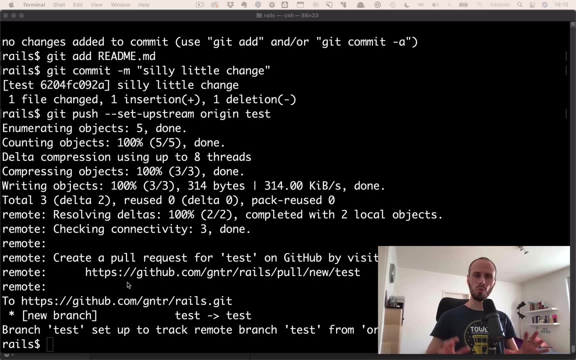 set up stream origin test And once this is available, okay, so this has worked. So we have now created the changes that we can request to be included. Once I've pushed them to my remote repository on GitHub, I can take another look at the. 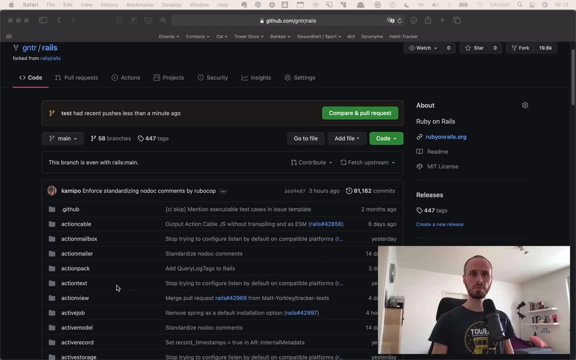 repository in the browser and see what happened. And voila, GitHub has noticed that I just pushed something here And since it's a fork, a forked repository, GitHub detected my changes and automatically asks me if I want to create a pull request with those changes, Because in a forked 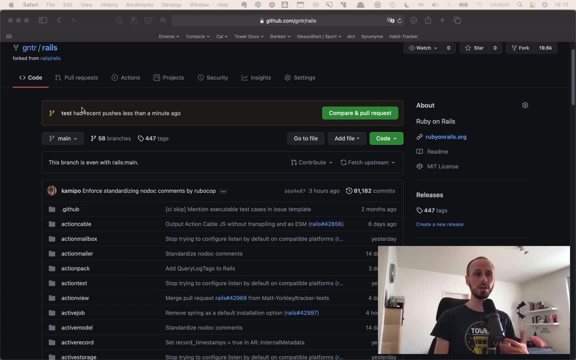 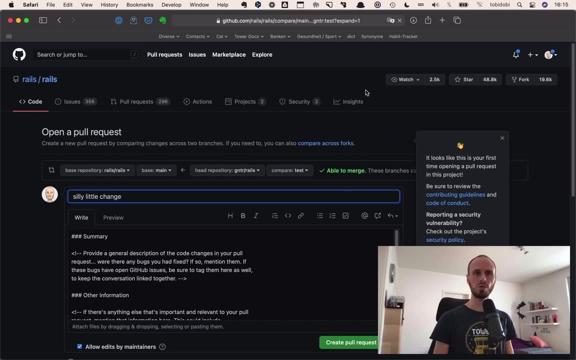 environment. this is mostly what you want to do, And if I do, I can propose which branch they should be integrated in. So I'll start the pull request process here. So at the moment I'm proposing to integrate my changes from my little branch here in the fork back into the main branch. 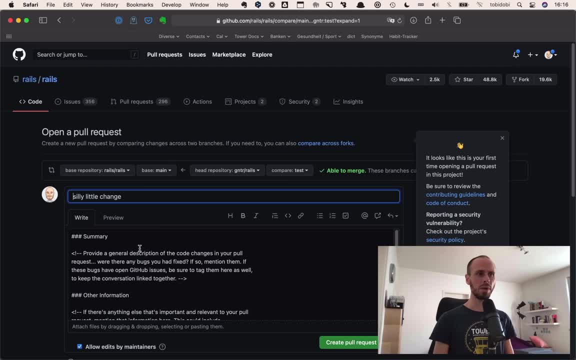 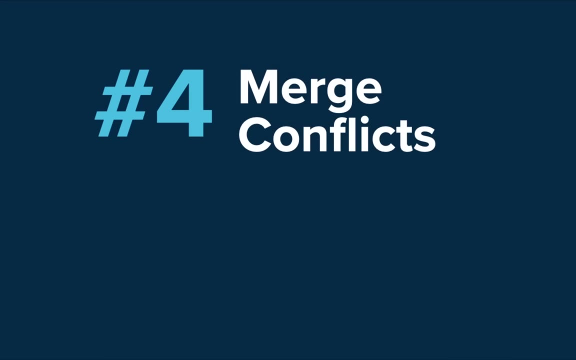 in Rails And let's say that is okay And I can add some comment And I could then create the pull request and the maintainer of the original repository would then be notified And they can review my changes and possibly integrate them. Merge conflicts: nobody likes them, but they are a fact of life when you're working with Git And in most 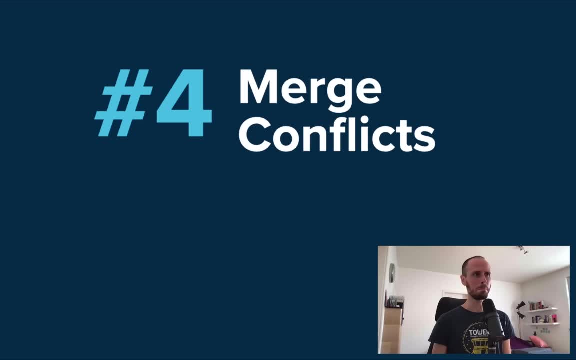 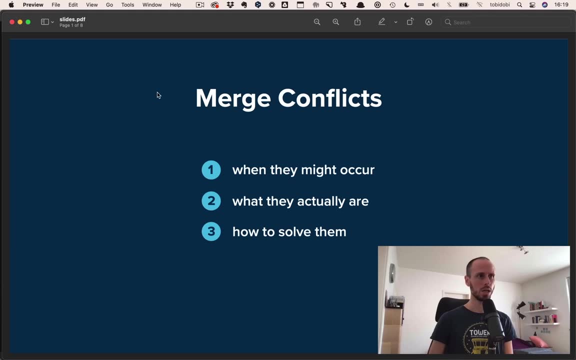 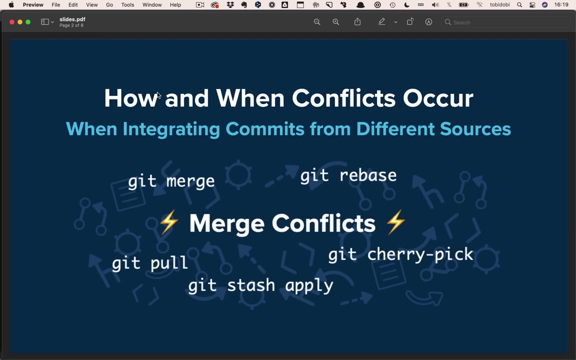 cases. they are not as tragic as we often think. We'll talk about when they happen, what they actually are and how to solve them. All right. So the name already says it: merge. conflicts can occur when you integrate, when you merge changes from a different source. 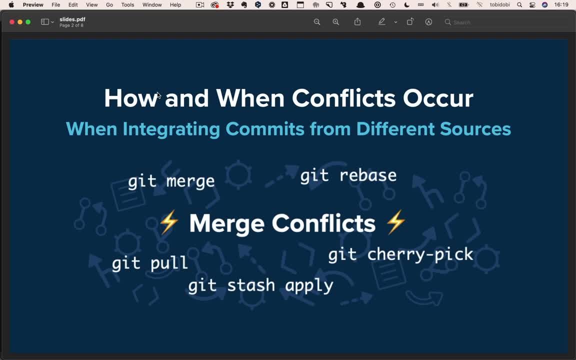 But keep in mind that integration is not limited to only merging branches. Conflicts can also happen when rebasing, interactive rebasing, when performing a cherry pick or a pull, or even when reapplying a stash. All of these actions perform some kind of integration, And that's when merge conflicts can. 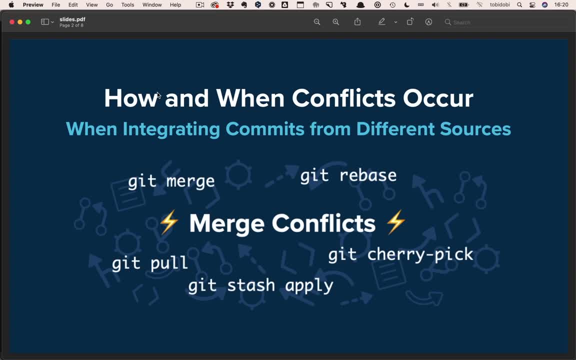 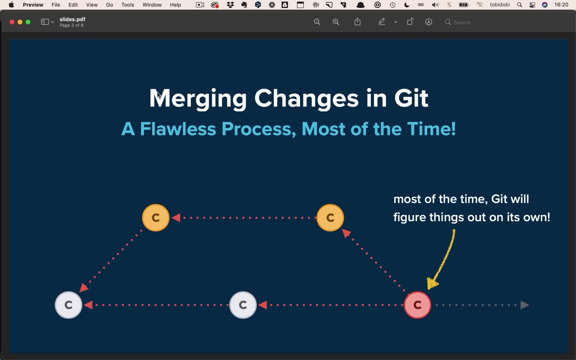 happen. Of course, these actions don't result in a merge conflict every time, thank God. But when exactly do conflicts occur? Actually, Git's merging capabilities are one of its greatest features and advantages. Merging branches works effortlessly most of the time because Git is usually able to figure things out. 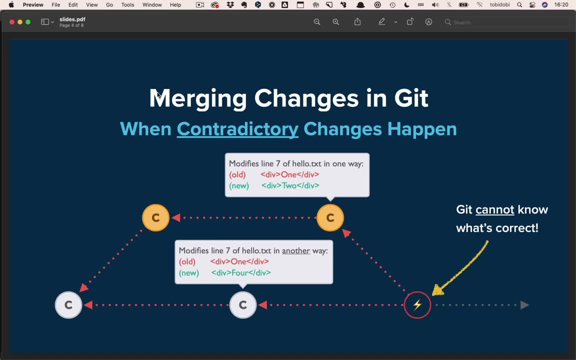 on its own. But there are situations where contradictory changes were made, And that's when technology simply cannot decide what's right or wrong. These situations require a decision from a human. The true classic is when the exact same line of conflict is made, And that's when the 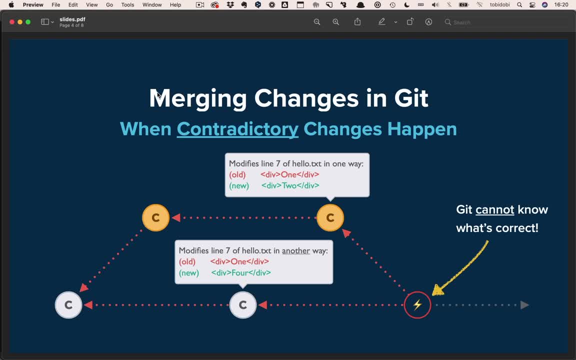 code was changed in two commits on two different branches. Git has no way of knowing which change you prefer. There are some other similar situations that are a little bit less common. For example, when a file was modified in one branch and deleted in another, But the the same. but the problem is: 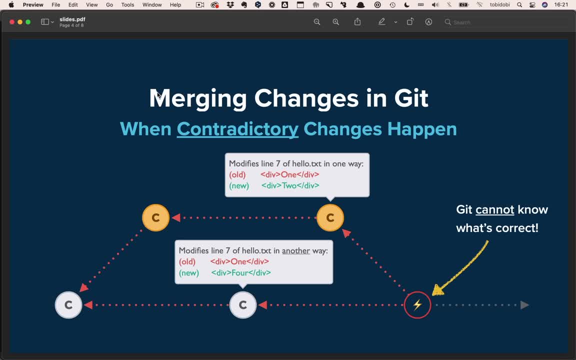 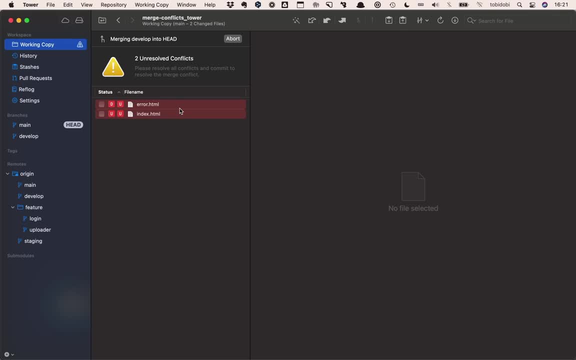 always the same Changes contradict. When you're working with a desktop GUI like tower, forget that can make things easier, especially because it's just more visual. I can select things here And this helps me understand what actually happened, So I can see these two changes conflict and I could select one or both or just this here. 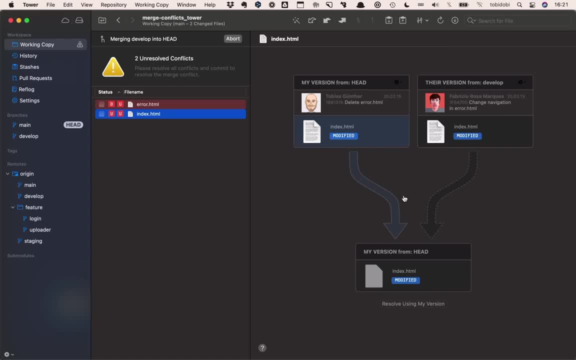 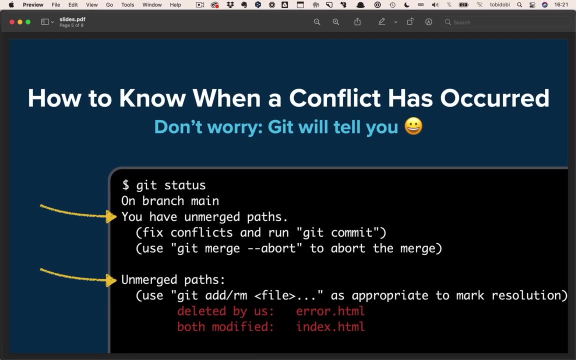 and solve the conflict pretty easily. How do you know when a conflict has occurred? Don't worry about that. Git will tell you very clearly when a conflict has happened First. it will let you know immediately in the situation, for example, when a merge or rebase fails with a conflict. So 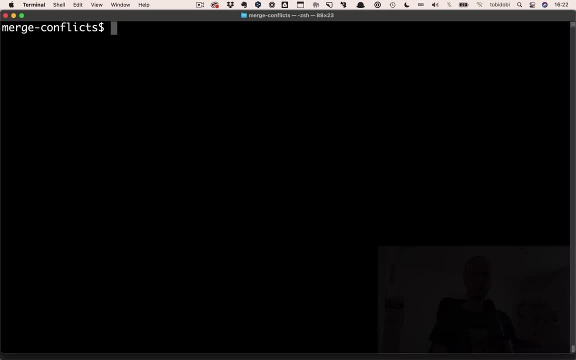 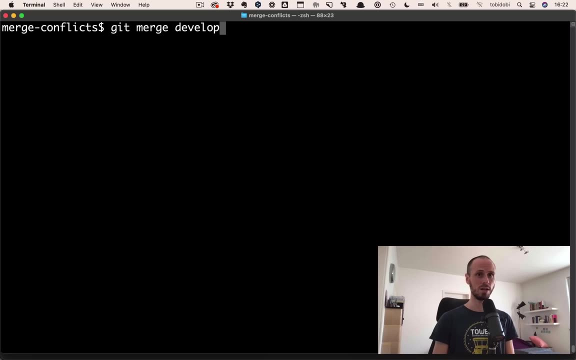 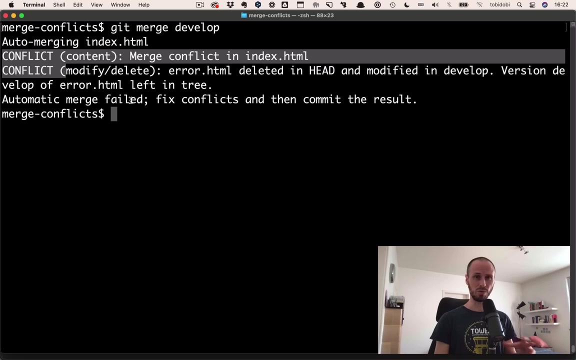 let's try this out. Actually, we have something here. let's provoke a merge conflict And I'll just try to merge in development to my main branch And voila, automatically. I can see something is wrong here: Conflict, conflict, conflict, automatic merge failed. So you can see that when I tried to perform the 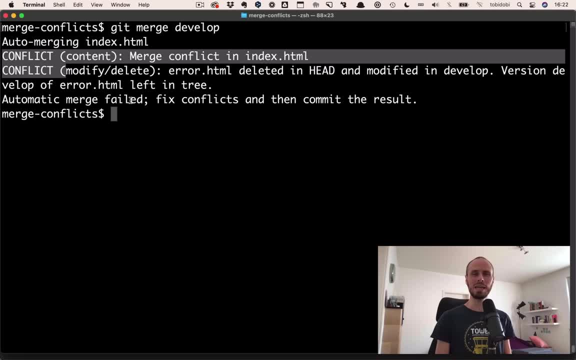 from the merge, I ran into conflict And it tells me instantaneously about the problem. But even well, even if I had overlooked these warning messages, I would find out about the conflict the next time I run- get status. So let's do that. 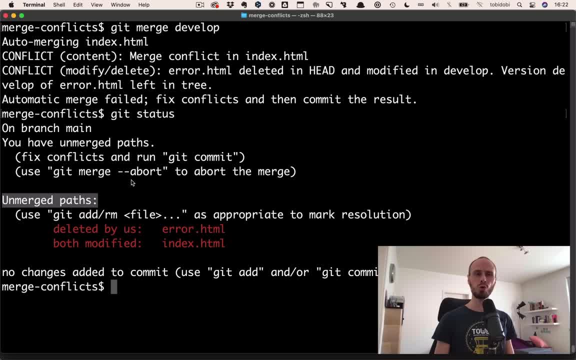 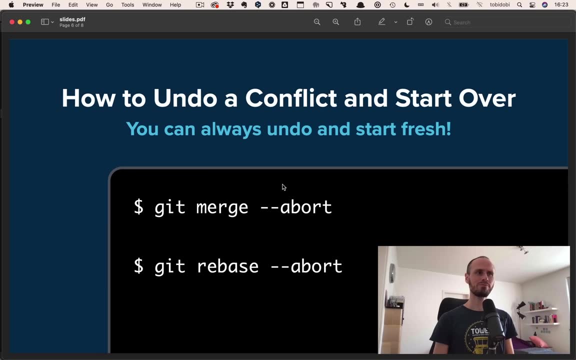 And pretty quickly you have this unmerged path category in the status here. So, in other words, don't worry about not noticing merge conflicts. get make sure you can't overlook them. All right, Though you can't ignore a merge conflict, you really have to deal with it before you can continue your. 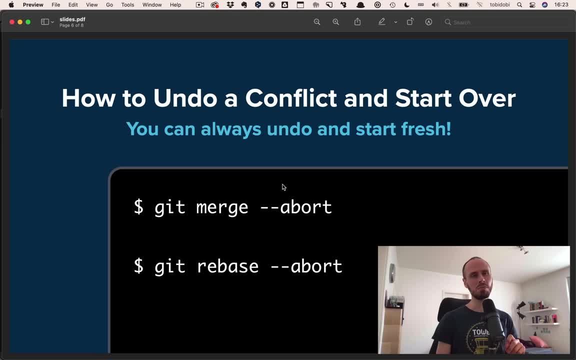 work. Dealing with a merge conflict doesn't necessarily mean you have to resolve it. you can also undo it, And this is sometimes very helpful. So keep this in mind always. you can always undo a merge conflict and return to the state. 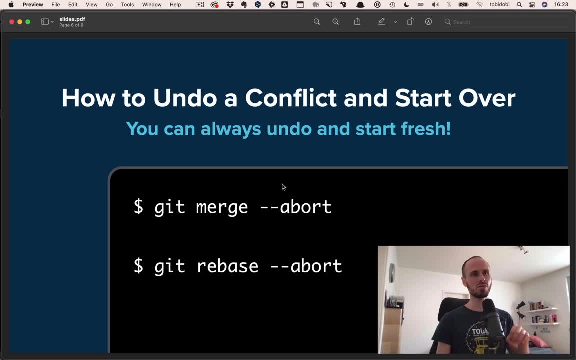 before you have a merge conflict Before. And this is true even when you've already started resolving some of the conflicted files and you notice, oh God, I'm, I'm on the wrong track here. Even then, when you find 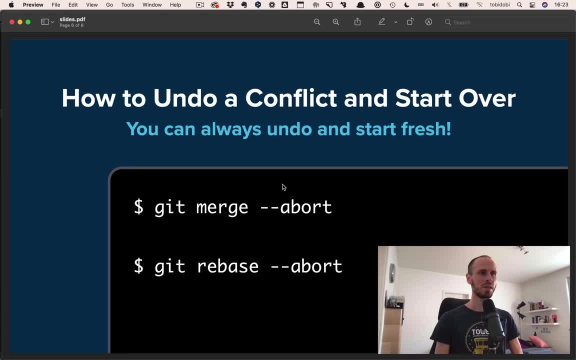 yourself in the dead end. you can still undo the merge, And some commands come with an abort option that lets you do exactly that. So the most prominent examples are git merge abort and git rebase abort. So in our example here, when I find why I 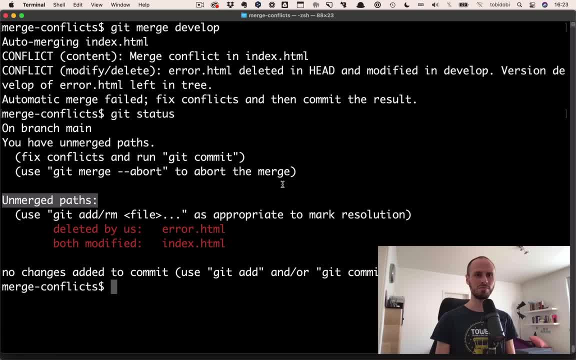 don't have the the time to deal with this right now or I've resolved something the wrong way. I can always type git merge, dash, dash, abort here And git status shows me I'm back to normal again. So this should give you the confidence that you really cannot mess up. you can. 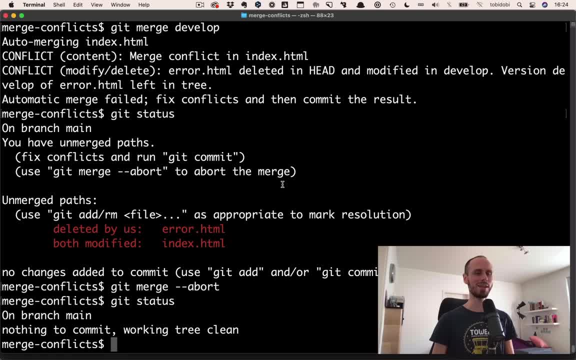 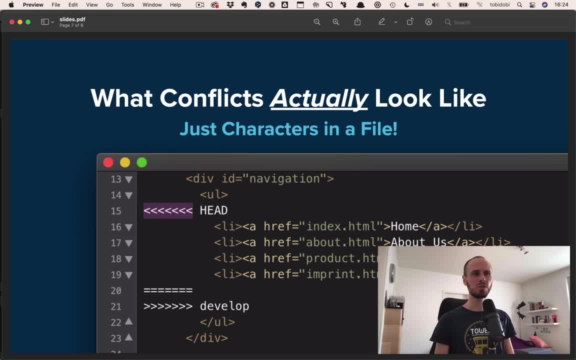 always abort, return to a clean state and try again, start over. So let's see what a conflict really looks like under the hood. we will demystify those little buggers and, at the same time, help you lose respect for them and gain a little bit of confidence. So as an example, 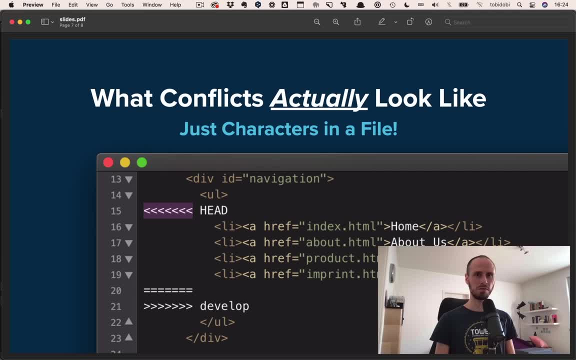 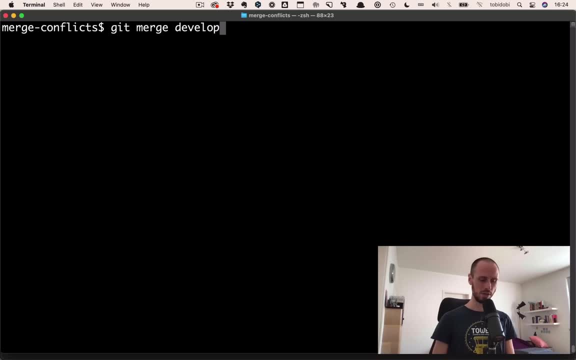 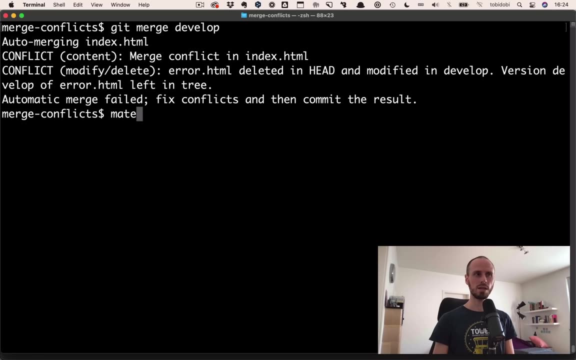 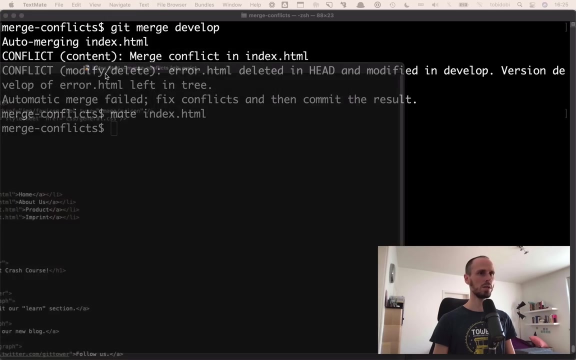 let's look at the contents of one of the conflicted files. I'll provoke that merge conflict once again, And I can see that in my index HTML file I have a conflict. So let's take a look at that. And nope, not this one, but this one. So get was kind. 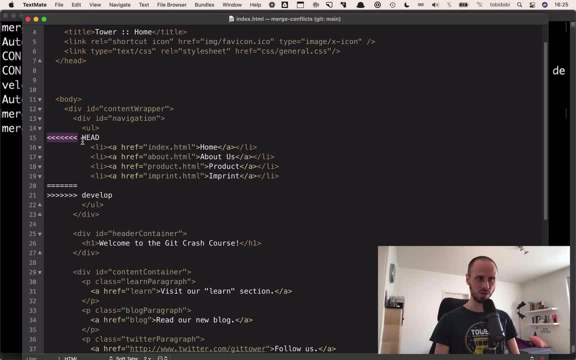 enough to mark the problematic areas in the file, So they're surrounded by these symbols here. this is the start and this is the end of the problem area. So the content that came- that comes after the first marker original- originates from our current working branch. 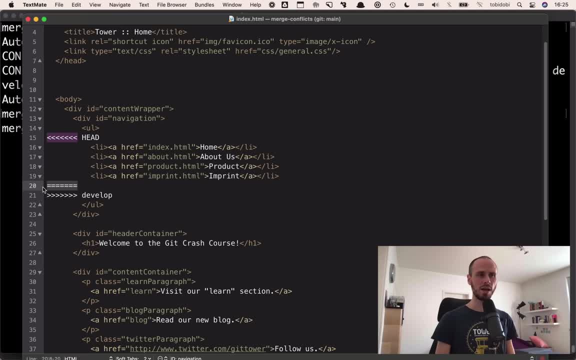 And then align with some equal lines, equal signs, separates the two conflicting changes. And finally, this here came from the other branch that's displayed as well. So in this case it's pretty simple. In the develop branch, where I made some 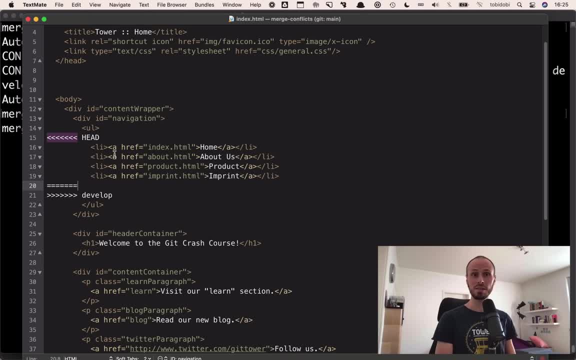 changes. I deleted this list item, these list items, And in my head branch I changed them. So git is unsure. did you want to change them like like this, Or did you want to delete them Like here? and I have to tell git what's correct and what's not. 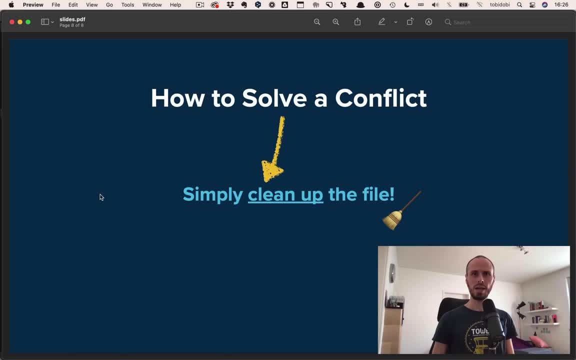 Okay, so how can you solve a conflict? Solving a conflict is actually pretty simple. we need to clean up these lines And after we're finished, the file should look exactly as we want it to look. So it might be necessary to talk to the 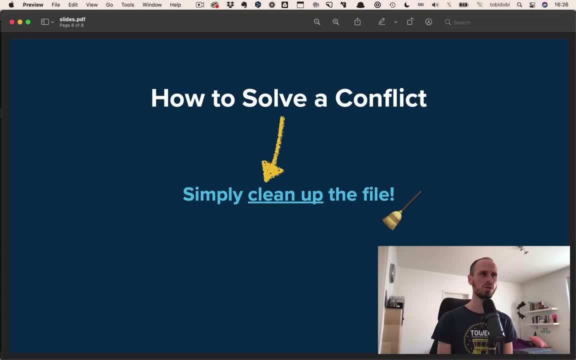 teammate who wrote the other changes and decide which code is actually correct- Maybe it's ours, maybe it's theirs, maybe it's a mixture between the two- And this process of cleaning up the file, making sure it contains the what we actually want. This doesn't have to involve any. 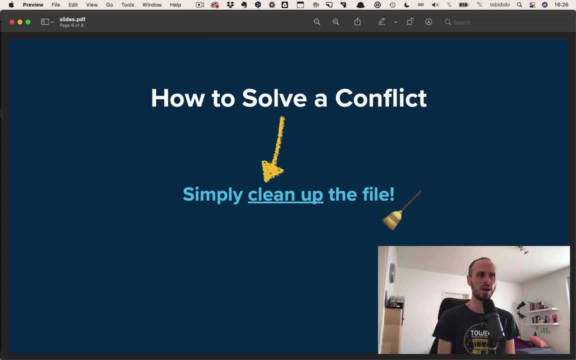 magic. you can do this simply by opening your text editor or IDE and make some changes. Sometimes, though, you'll find that this is not the most efficient way. That's when dedicated tools can save you a little bit time and effort. So 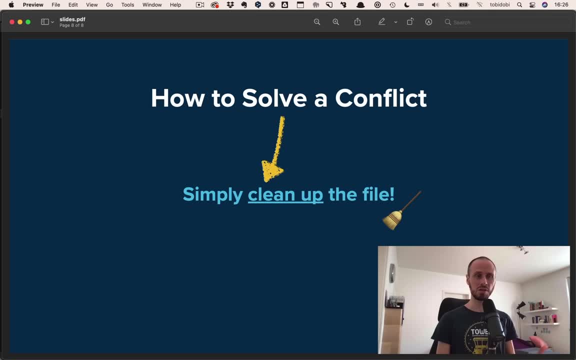 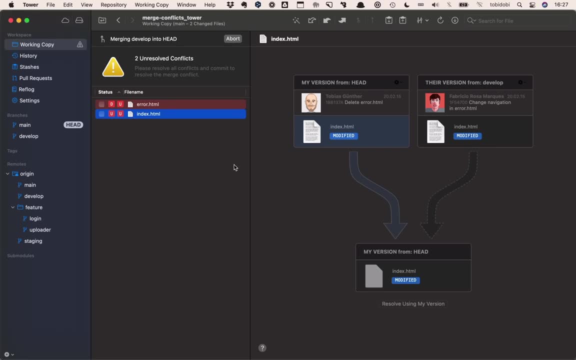 on the one hand, there are git desktop GUIs. some of the graphical user interfaces for git can be helpful when solving conflicts. you've already seen one, So this is tower where you could, where you can see what happened in the conflict, And 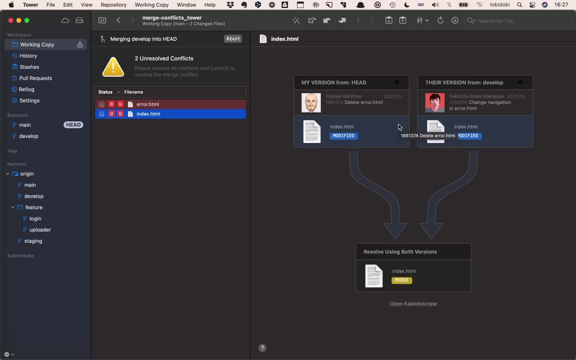 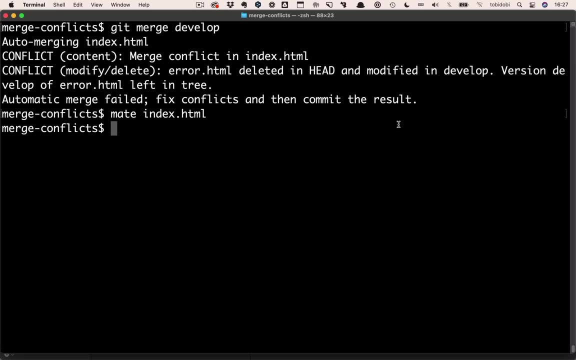 this visualizes the problem And, on the other hand, there are dedicated merge tools for more complicated conflicts and can be great to have a dedicated, different merge tool at hand. you can configure your tool of choice using the git config command And then, in case of a conflict, you can simply type: 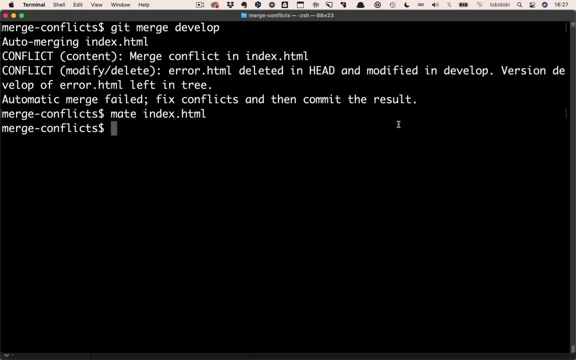 git merge tool and have it open the conflict. I have a kaleidoscope app installed on my Mac, So let's just try this git merge tool. I configured that. So the first one, as you can see, is pretty easy. One of the second one. 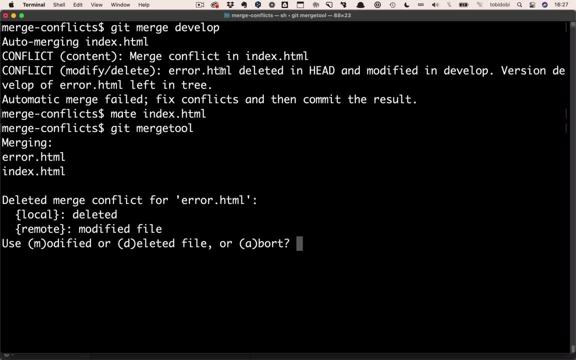 here. our HTML was deleted, So I don't need to see that. I just need to decide: do I want to keep it or do I want to delete it? So I'll stick with the deletion. And for the second one, there's really content in the file where it makes sense to. 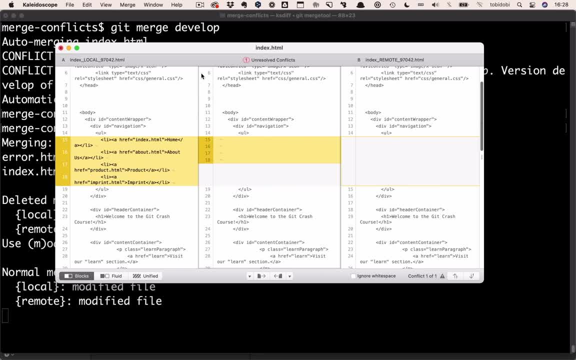 open that merge tool that I configured, I can see: well, this is the change that I made And this is the change that came from another person or from a different branch. And what do I want to look like? what I want it to look like, I can choose. 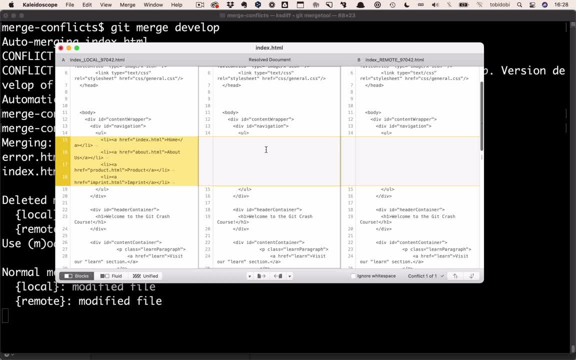 these changes or these here, or can make my own changes here. So, after cleaning up the file, either manually or in a desktop, do we agree or merge tool? I have to commit this like any other change, So I can save it here and say this is resolved, And if I type git status, I can 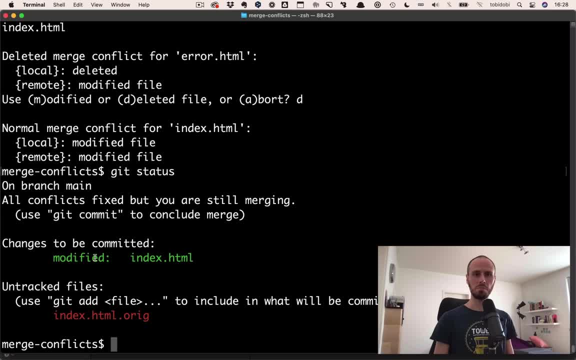 see these changes would be committed. I made some changes here in index HTML. this here is just a safety copy. you can configure that also to to happen, So you can always return to the, to the original file. But I would actually just commit this: 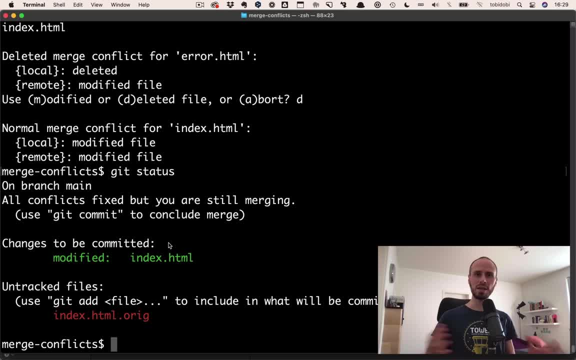 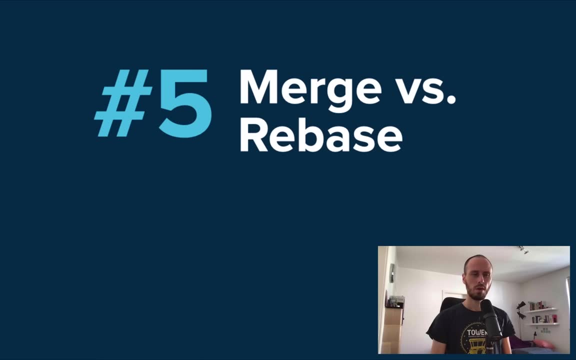 here And simply by committing the resolved files I signal to get that conflict is completed And I can go on with my work. Most developers understand that it's important to use branches in Git, because having separate containers for your work is incredibly helpful. Let's talk a bit about integrating branches. 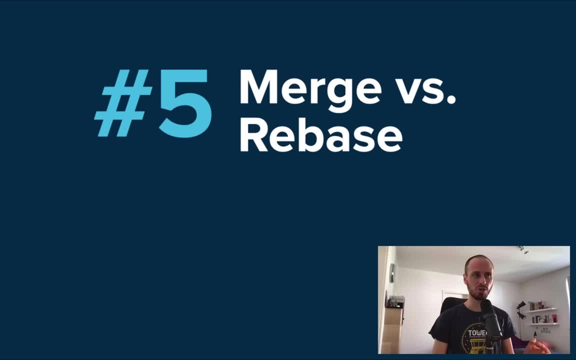 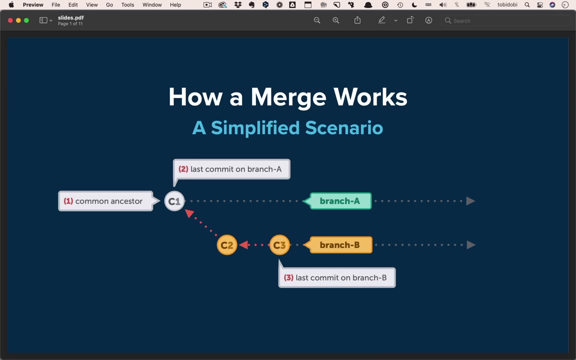 about your new code back into an existing branch. There are different ways to do this, And the two most common ones are merge and rebase. Let's start by talking about merge and how it actually works. When Git performs a merge, it looks for three commits. 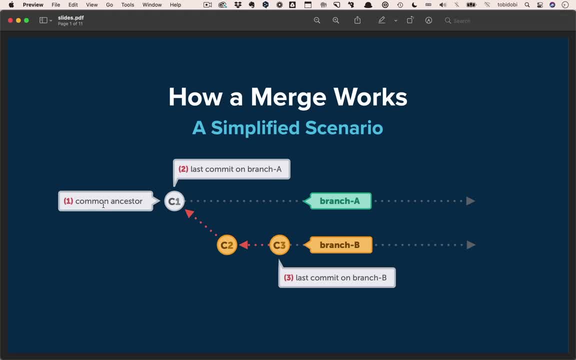 First, the common ancestor, commit. If you follow the history of two branches in a project, they always have at least one commit in common. At this point both branches have the same content And after that they evolve differently. The other interesting. 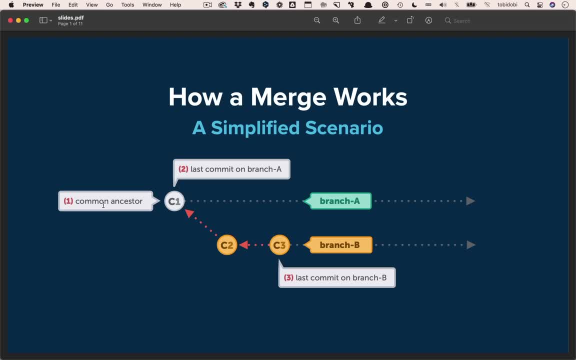 commits are the endpoints of each branch. Remember that the goal of an integration is to combine the current states of two branches, So the latest revisions are, of course, important. Combining these three commits will perform the integration that we're aiming for. I've chosen a very simple. 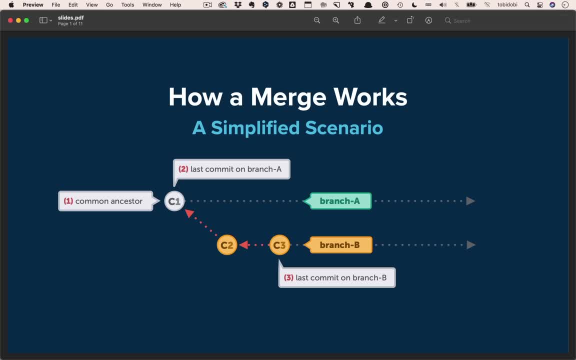 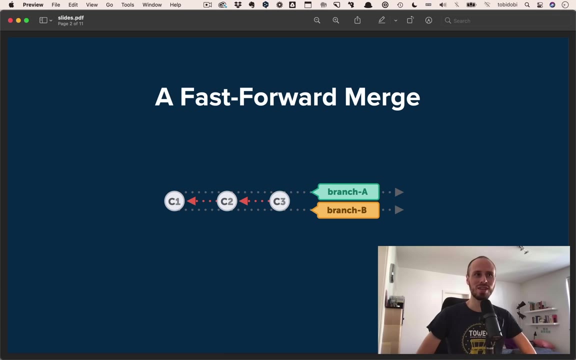 example case here. because one of the two branches are branch A here, It didn't receive any new commits after the branching happened, So its latest commit is also the common ancestor. In this case the integration is dead simple. Git can just add all. 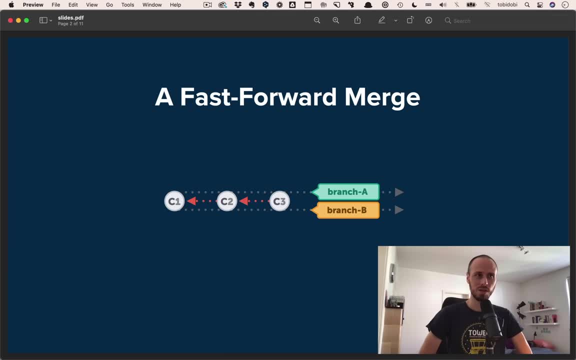 the new commits from branch B on top of the common ancestor commit, And in Git the simplest form of integration is called a fast forward merge. Both branches then share the exact same history. In most, most cases, however, both branches move forward differently. 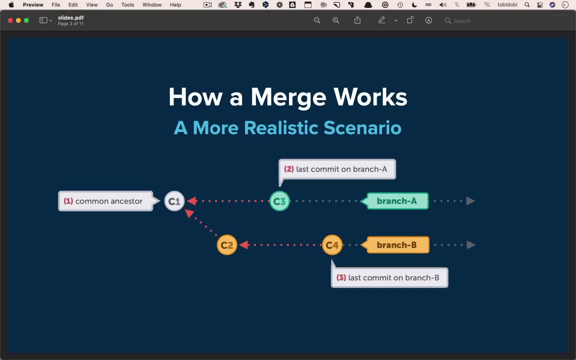 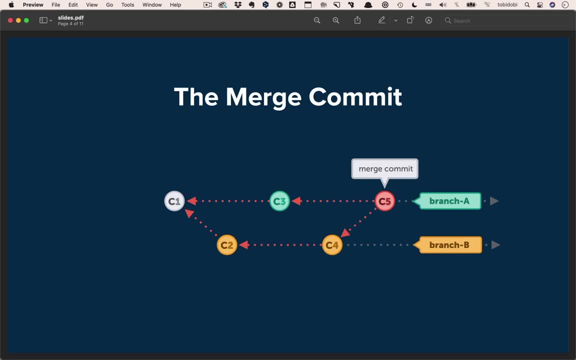 of course, And to make an integration, Git will have to create a new commit that contains the differences between them, And this is what we call a merge commit. Normally, a commit is carefully created by a human being. It's a meaningful unit that wraps only related changes and the commit message provides. 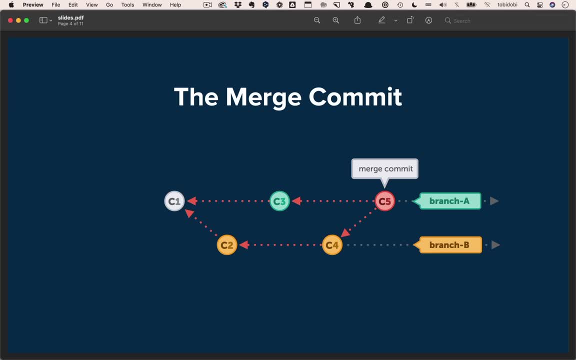 context and notes. Now, a merge commit is a bit different. It's not created by a kleinados in its own election. the merge outcome is a by a developer. it gets created automatically by Git And it also does not wrap a set of related 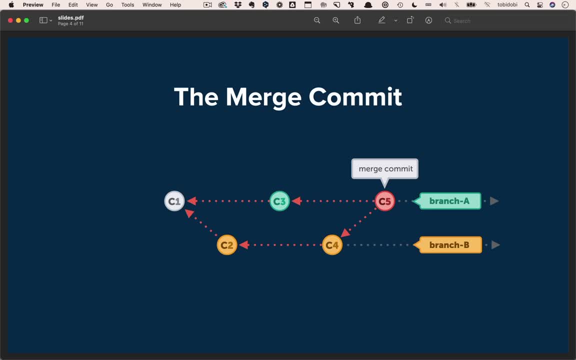 changes. Its purpose is to connect two branches just like a knot. If you want to understand a merge operation after the fact, you need to take a look at the history of both branches and their commit history. Now let's talk about rebase, But before we start, let me emphasize: 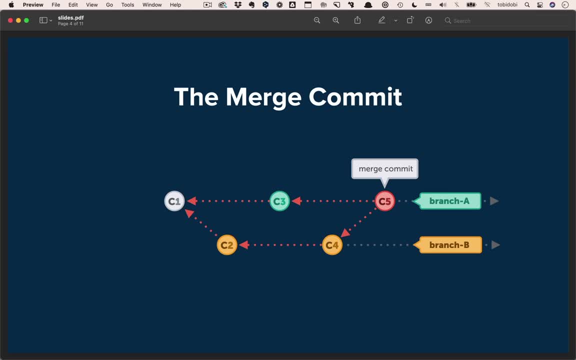 something. rebase is not better or worse than merge. Most importantly, it's different. You can live a happy Git life just using merge, But rebase has its pros and cons. So knowing what it does and when it could be helpful is nice. All right, Remember that we just talked about the automatic. 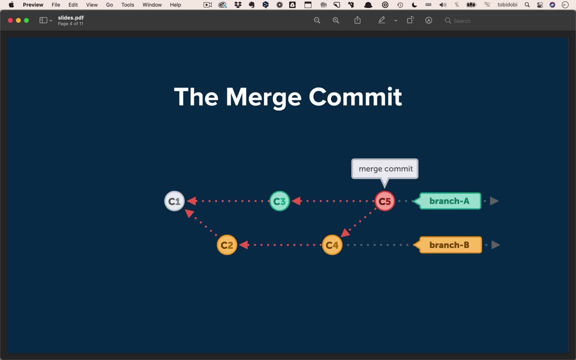 merge, commit. Some people would prefer to go without these. They want the project history to look like a straight line, without any signs that it had been split into multiple branches at some point, even after branches have been integrated. And this is what happens with rebase. 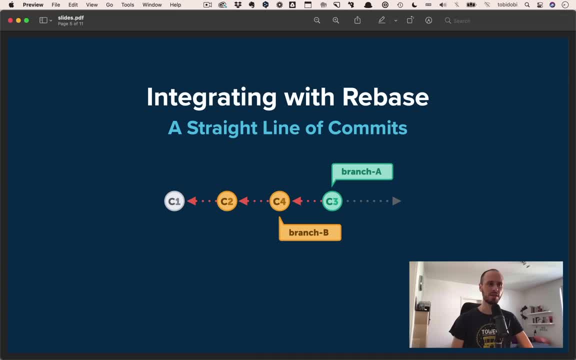 Let's walk through rebase operations step by step. The scenario is the same as in the previous example. we want to integrate changes from branch B into branch A, But now by using rebase, the actual Git command, to start. this is really simple. It's just Git, rebase And the branch 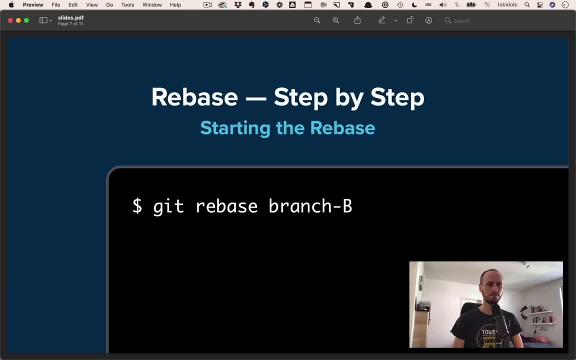 similar to the previous example, we want to integrate changes from branch B into branch A. Similar to the previous example, we want to integrate changes from branch B into branch A. we just tell Git which branch we want to integrate. But let's take a look behind the 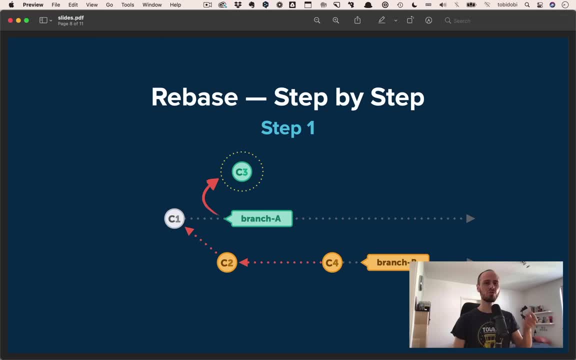 scenes. First, Git will remove all commits on branch A. that happened after the common ancestor commit. But don't worry, it will not throw them away. You can think of those commits as being parked, as saved somewhere temporarily. Then Git applies the new commits from branch B. 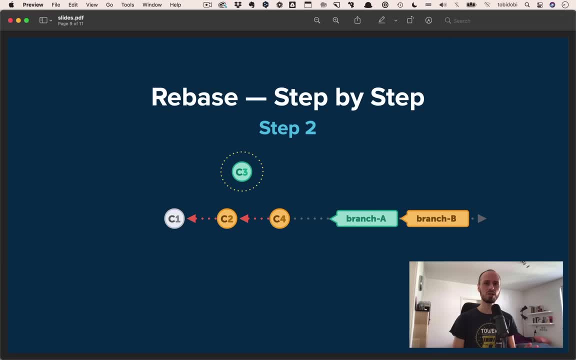 And at this point, temporarily, both branches look exactly the same, But in the final step those parked commits need to be included, The new commits from branch A. they're positioned on top of the integrated commits from branch B. they are rebased. 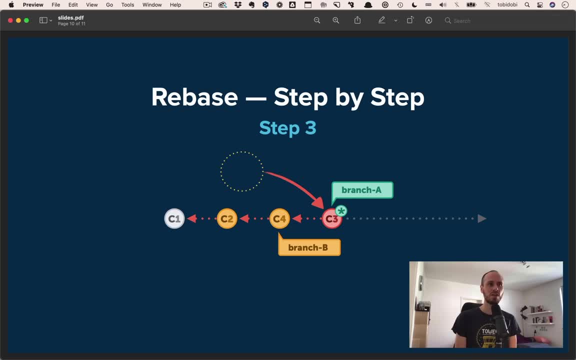 as you can see, And the result looks like development had happened in a straight line. There's no merge commit that contains all the combined changes. We preserved the original commits from branch B as well, And today I'll go over a separate slide in the future. But let's 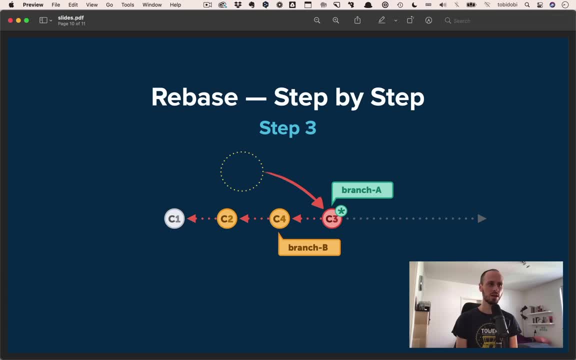 talk about how to add a new commit to your package. After that, we need to add a new commit In the same way that we did with the initial summary. we have to add a new commit that contains both the same contents of the first and last constructor, In the same way. 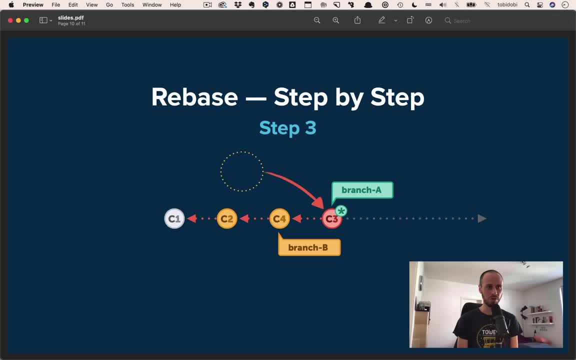 that we did with the initial summary. So there's a new commit that contains all the elements already based on two. A commit has only a handful of important properties, like the author date change set and who its parent commit is, And changing any of this information effectively. 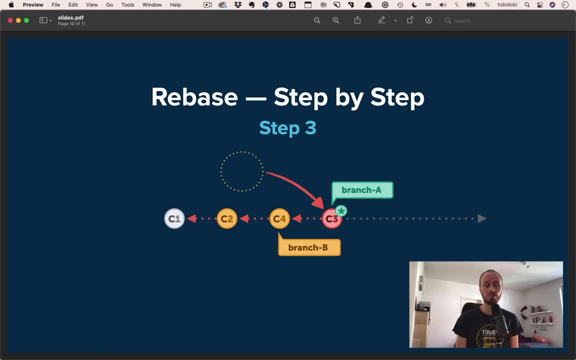 creates a completely new commit and with a new commit hash. So rewriting history like that is not a problem for commits that haven't been published or pushed yet. But if you're rewriting commits that have already been pushed to a remote repository you might be in trouble because 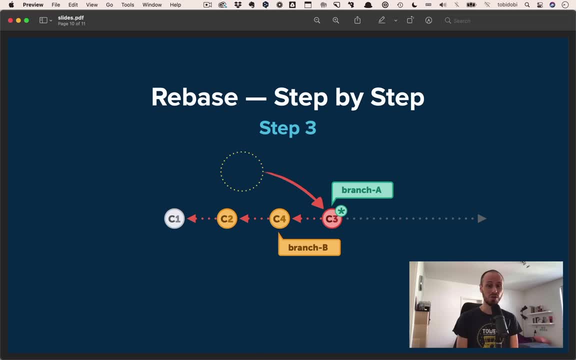 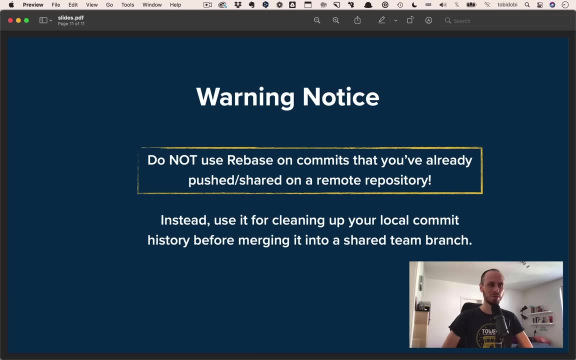 another developer might have based their work on the original C3 commit, which is not here anymore. So let's close this topic with a simple rule: Do not rewrite commits that you've already pushed to a shared repository- Tools like rebase. you should only use them for cleaning up your local.